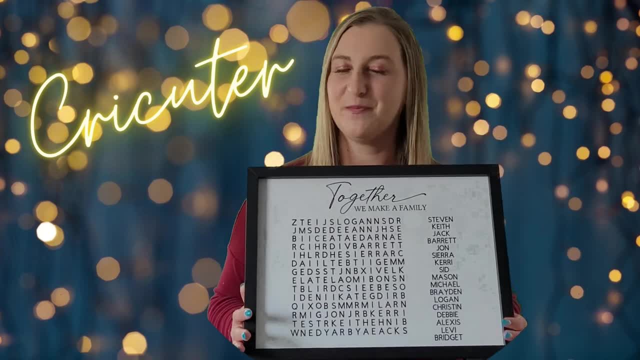 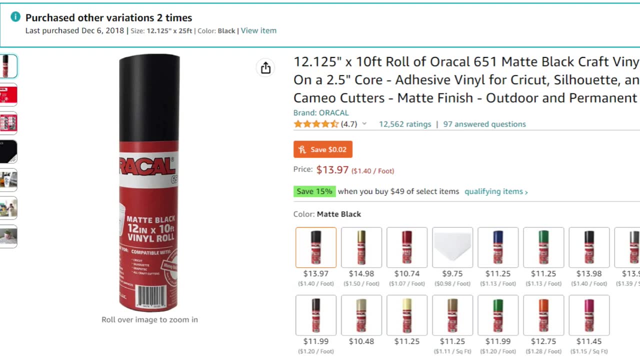 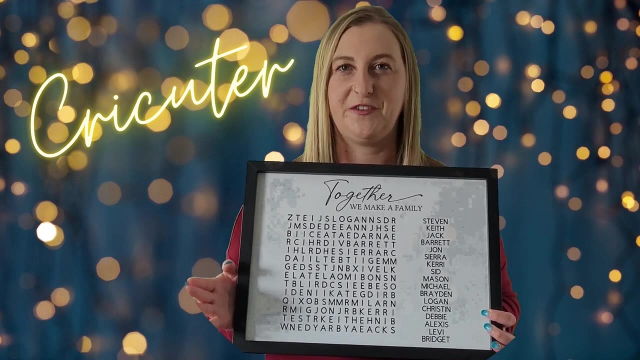 you need a dry erase board which is from Five Below. You also need vinyl. I definitely recommend using Oracle 651 vinyl. This is in the matte finish, not the glossy finish. It's really important to use high quality materials. The only kind of vinyl that I buy is Oracle 651.. You can get it anywhere. 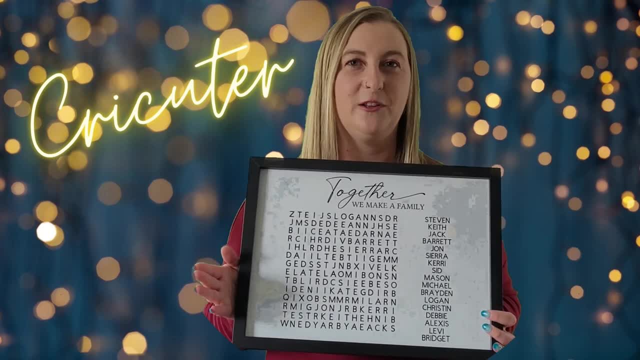 You can usually buy it on Amazon. I always buy black and white in the largest rolls possible, because those are the colors that I use most of the time on all of my cricket projects. If you know that you have a lot of vinyl, you can buy it on Amazon. You can buy it on Amazon, You can buy. a lot of vinyl to buy at once and it's going to be over $50.. I would recommend getting your vinyl from a website called 143 Vinyl. They have amazing prices, super fast shipping and free shipping over $50.. So that's why I said, if you have to spend over $50, I'd recommend getting your vinyl from. 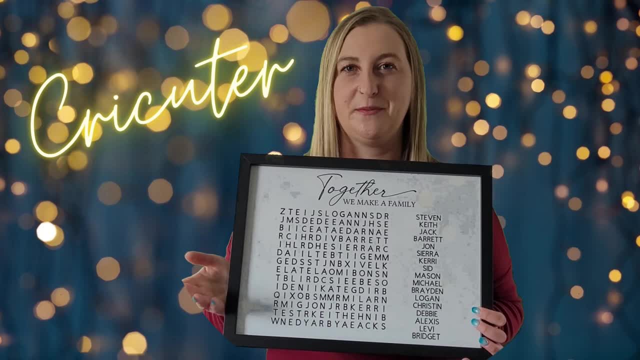 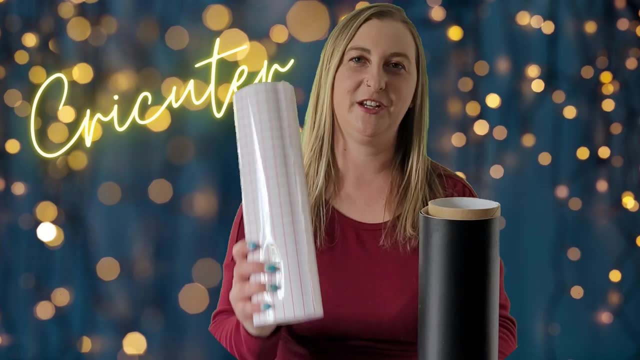 there. If you're spending less than $50, then just get it from Amazon or Expressions Vinyl or anywhere else where you choose to get your vinyl. I have my big roll of black Oracle 651.. You'll also need transfer tape. This is the best way to get your vinyl from Amazon. You can get it from 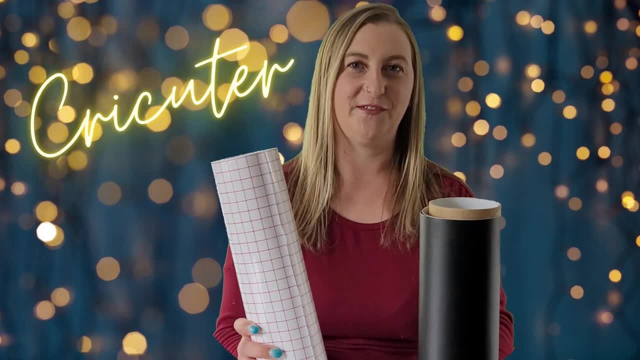 Expressions, Vinyl or anywhere else where you choose to get your vinyl from. This is the best transfer tape that I have ever used. I've tried a whole bunch of different ones. I found that the dollar store contact paper isn't sticky enough. Then for a while I was using a different kind. 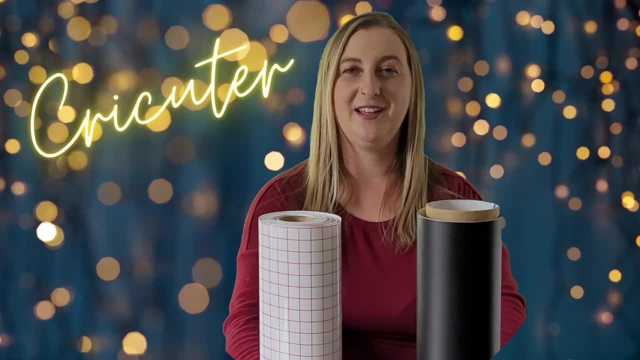 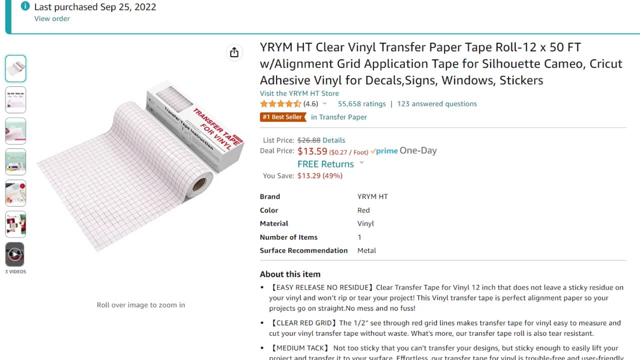 called Frasco, I think, and that one was way too sticky. This one is just right. I'll leave a link down below in my video description If you want to buy it. I got it right on Amazon. Some other tools that I would recommend using for this project is isopropyl alcohol and a coffee filter. 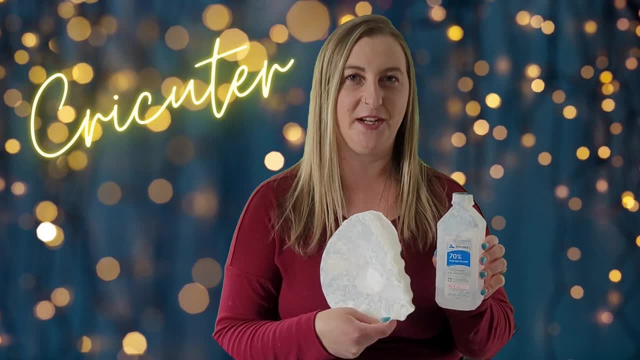 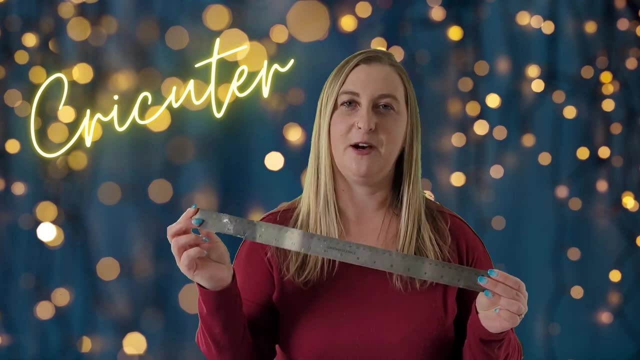 I use this to clean my blanks so that white part on your dry erase board you want to clean that before you apply your vinyl. I use a ruler to measure the white part on my dry erase board to see how big to make my design. I also use my Cricut cutter to 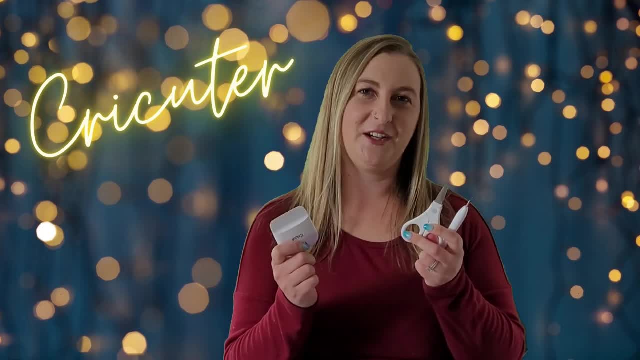 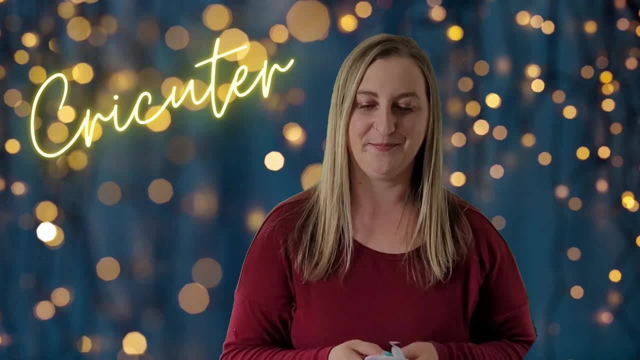 cut out my vinyl to the right size And, of course, some basic Cricut tools like your weeding pen, your scissors and your scraper, your spatula, whatever you call it, And then you'll need a Cricut machine. I would recommend using either the Cricut Explore Air 2, the Cricut Explore 3,. 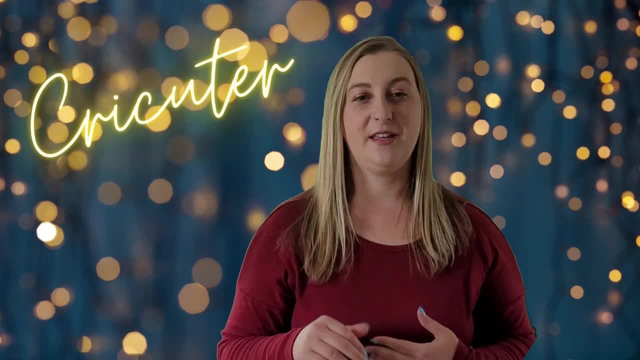 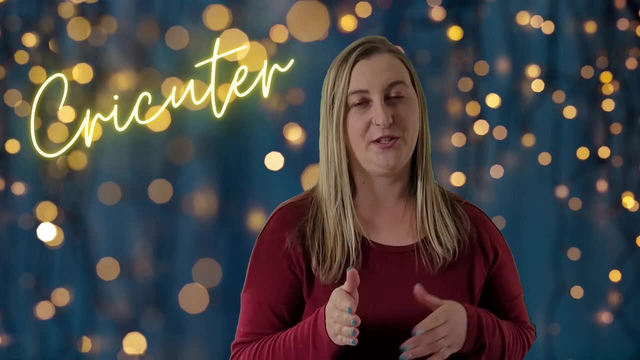 the Cricut Maker or the Cricut Maker 3.. This project you can't do on a Cricut Joy, because a Cricut Joy only cuts like four and a half inches wide. This project was almost 10 inches by 14 inches, So you need the. 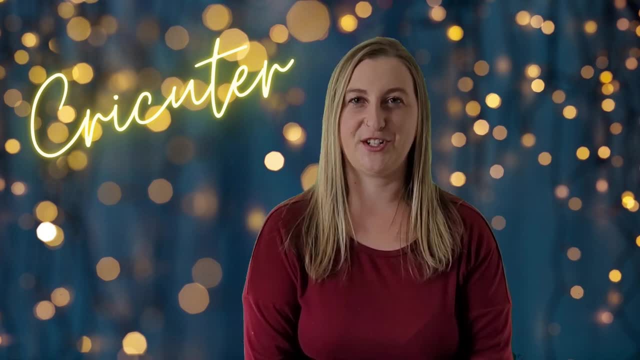 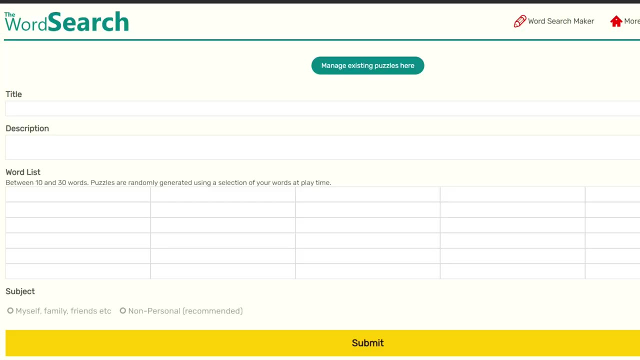 bigger machines from the Explore or the Maker series to make this project. I'm using a Cricut Maker And you'll also need a Cricut mat. I'm using the standard grip mat. I tried out a few different word search generators and I think that this one is the best. It's from thewordsearchcom. 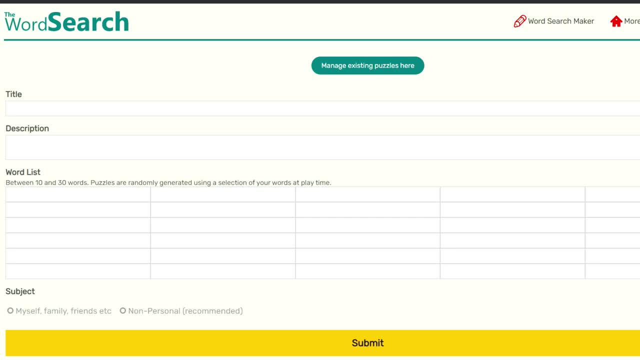 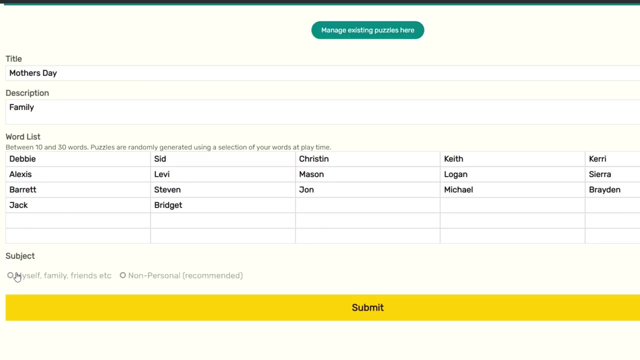 I'll leave a link down below in my video description. They make you put a title and description: Mother's Day. We'll just write family And this is where you type in all of the names. Once you have all your names put in, you select either this or this. 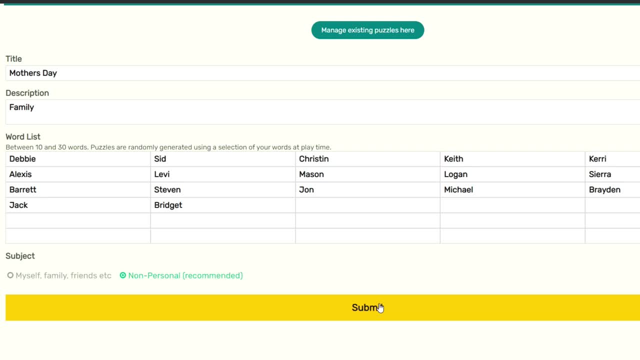 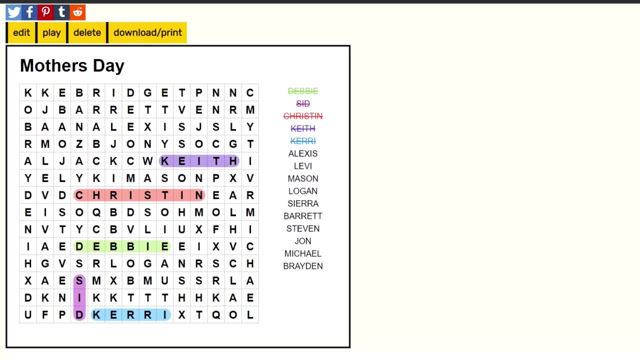 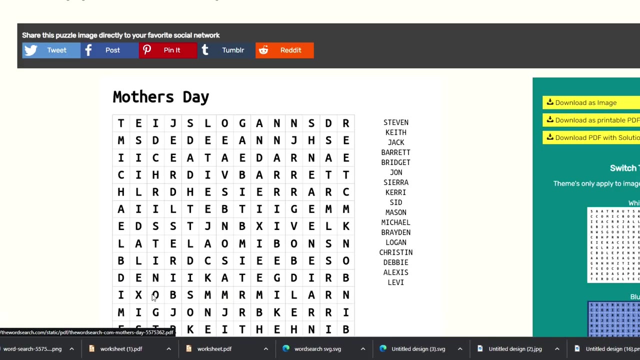 I don't really know what the difference is, but I just went with non-personal and we're gonna click Submit And then it gives you this really neat preview. So I'm gonna go ahead and click download slash print And I'm gonna download as image and just save it to my computer. 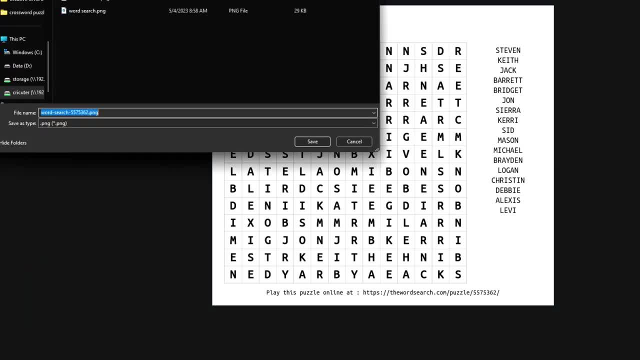 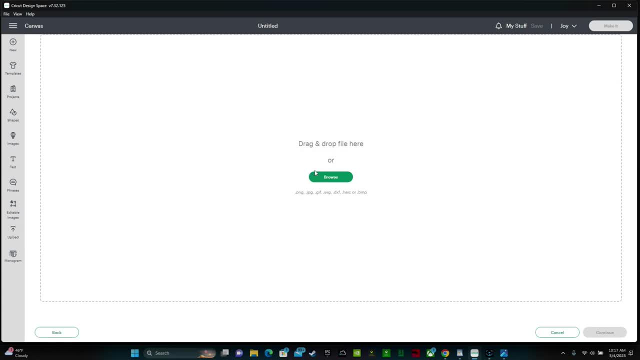 So right, click Save as And click Save Next. you want to go to upload, Upload image, Browse And select your file and click open. You want to click simple and then continue. First, I'm going to show you the way that you would think that you should do this. 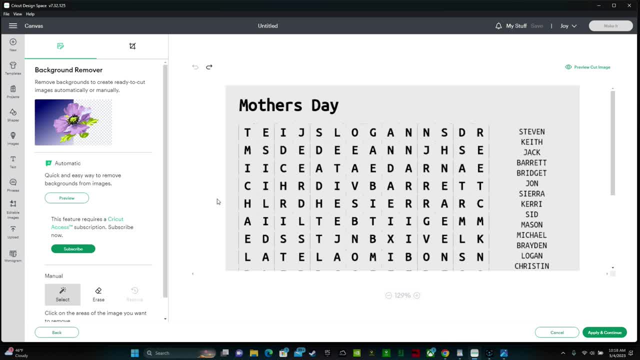 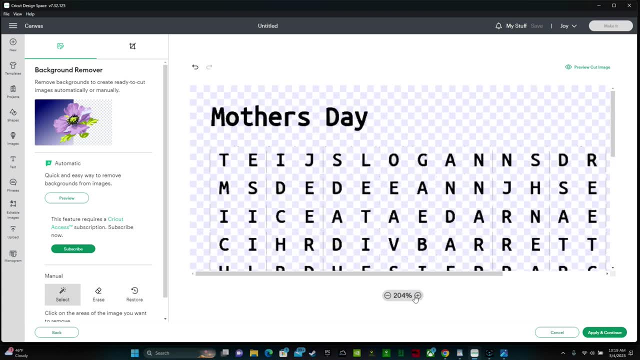 do this, and then i'm going to show you what i actually do and explain why. so common sense would tell you to use the select button and click here, and then zoom in and get rid of all of these little spaces in between the letters. i did that and it takes forever and the time isn't really. 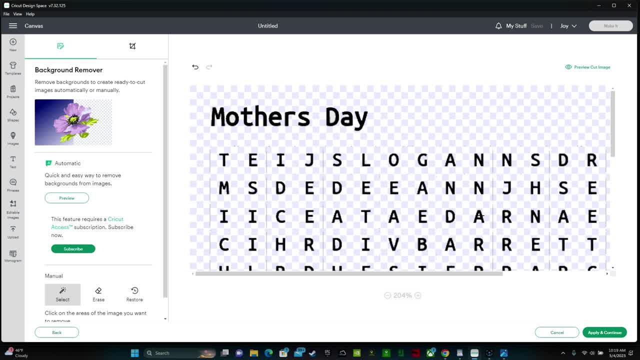 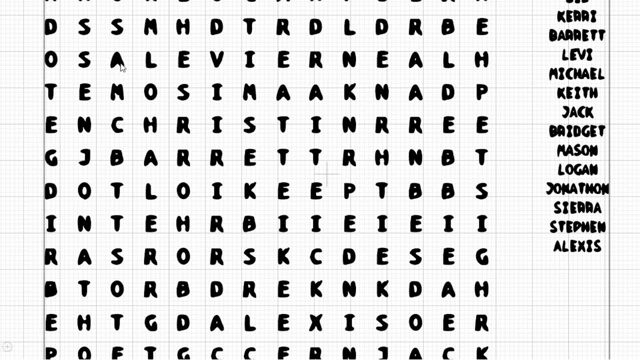 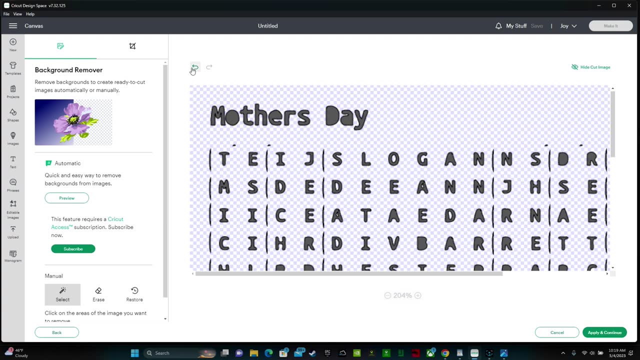 the problem. the problem is that the letters come out really blurry. i'll show you so we can click preview, cut image, and i only did a couple of letters, but you can see how they look like really bubbly and not like crisp letters. i hate that. so we're gonna go to the back button and we're just 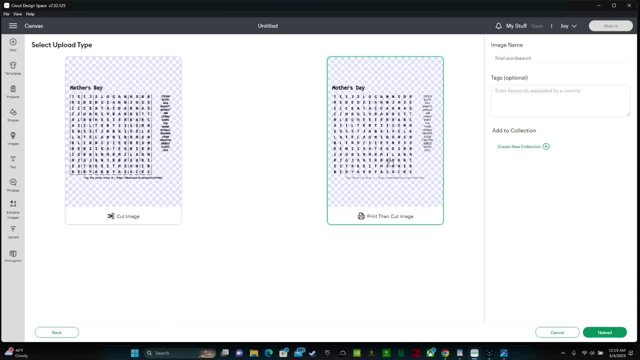 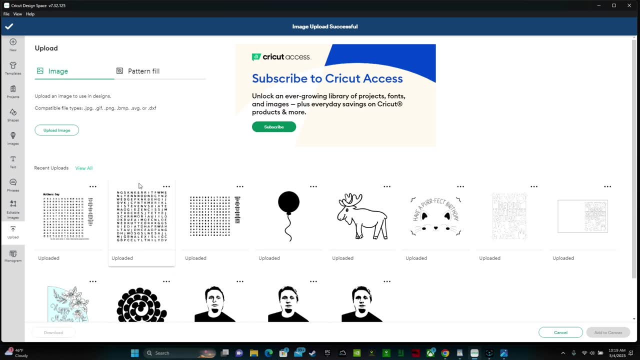 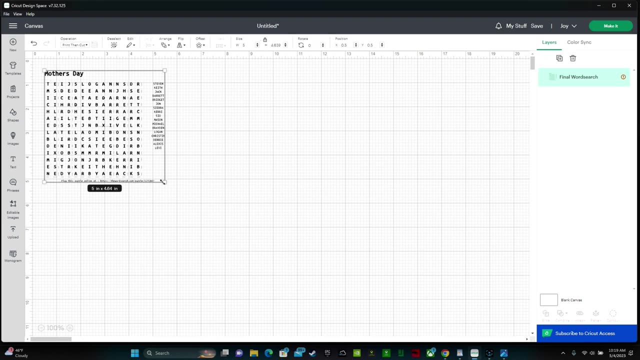 gonna click apply and continue and i'm gonna save it as a print, then cut image and click upload. we're not doing a cut image and don't freak out because we're not actually doing a print then cut. so basically what i wanted was just a template that i could see where the letters are. but i'm 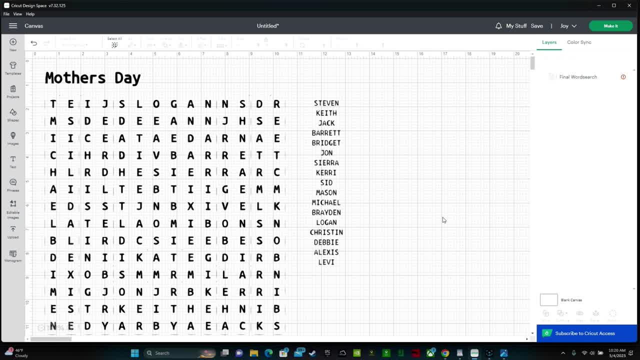 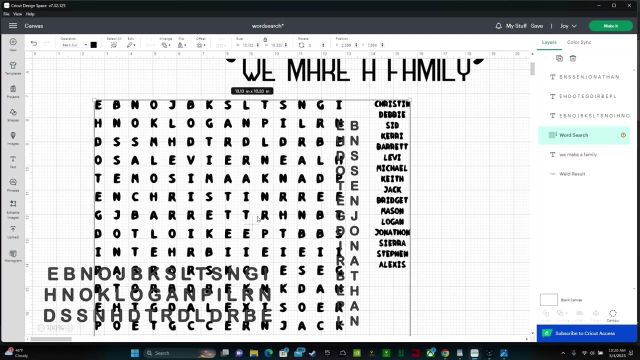 actually going to manually type them by hand in design space and you need to type them out in columns, so going up and down and not across, and i'll show you why. so i was playing around with this earlier and at first i uploaded it like this: where i went and i erased all of the spaces in. 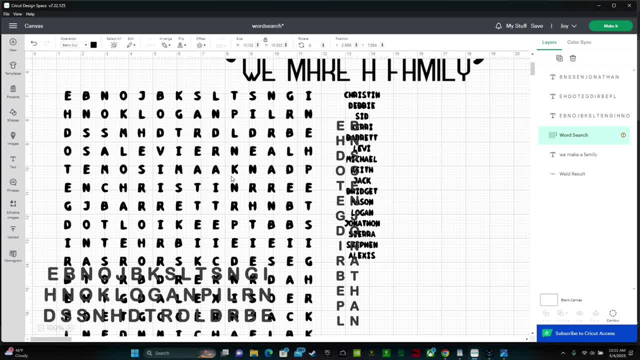 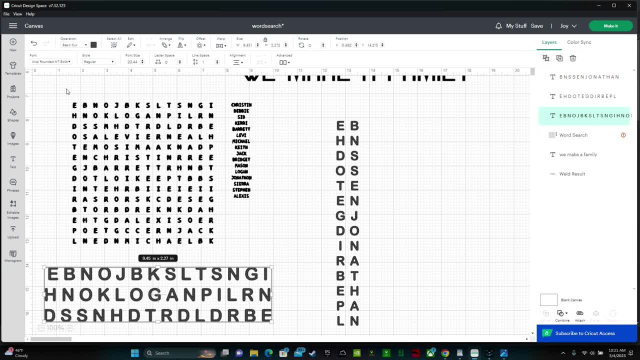 between the letters and you can see how they look all blurry and thick and not like crisp letters. so then i decided to try and type out all of these letters going across. so e, b and o, j, i did this row, then that row, then that row, and the problem is that these letters aren't lining up. 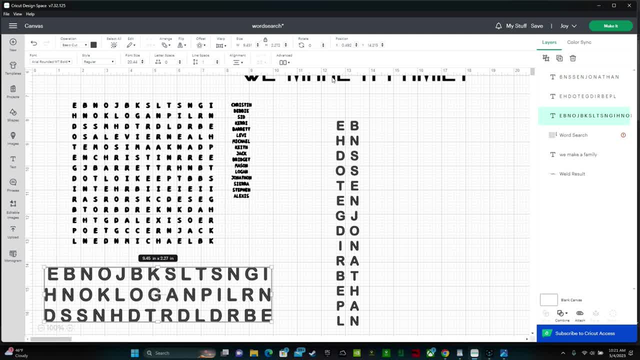 right. so then i decided to type in the letters and columns, and when i do them in columns, they end up in the right spots. so that's what we're going to do. we need to use this as a template and then type out the letters in columns all the way across. 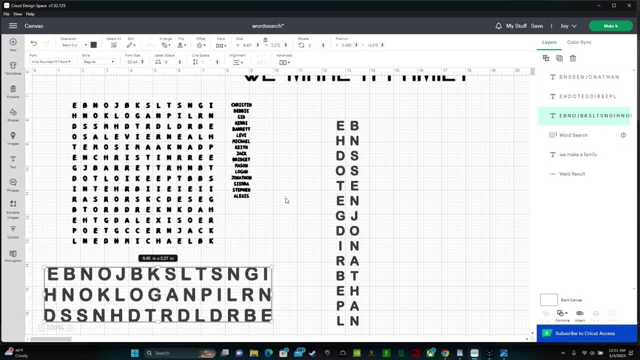 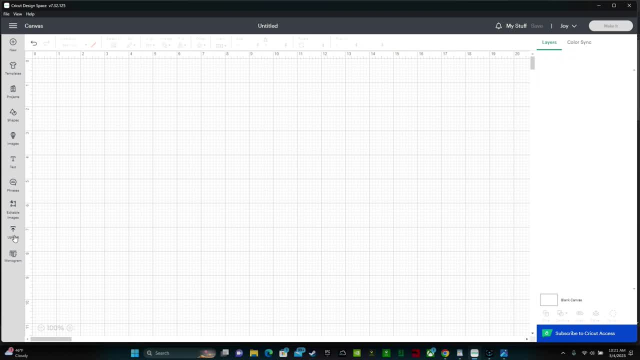 and then we'll retype out the names too. it's a little bit time consuming, but it's going to make this project come out perfect and the letters won't look weird at all. so back to our fresh new canvas. i'm going to go and click upload and select that file and click add to canvas. 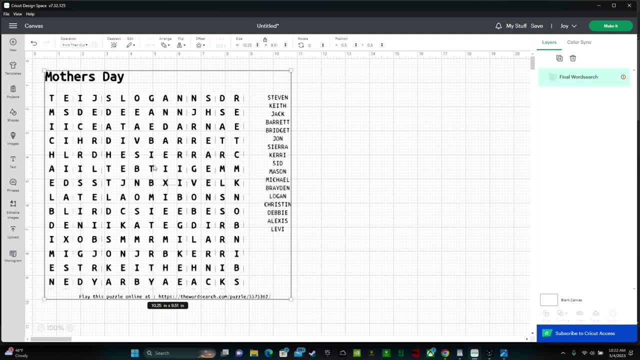 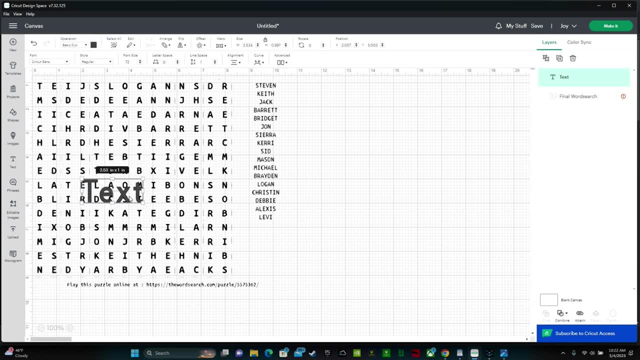 and i'm going to make it bigger so that i can see. now i'm going to click text and i want to move this text box over here and i'm going to type the letters i see going down. if we want to make sure that this is the same size as this, we can click it. 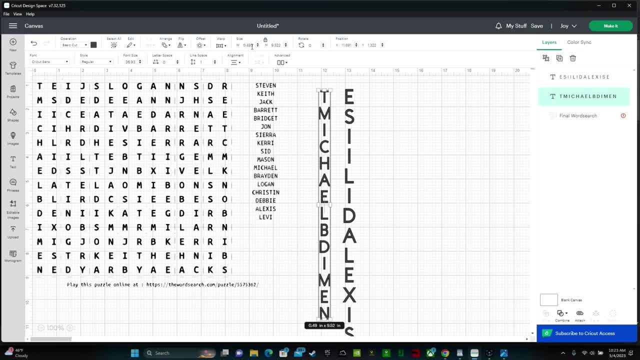 and look at the size. right here it says 0.493. so for simplicity, let's make it zero, 0.5 and click enter. and then this one: we can click 0.5 enter. this is 0.5 by 9.656, so let's make. 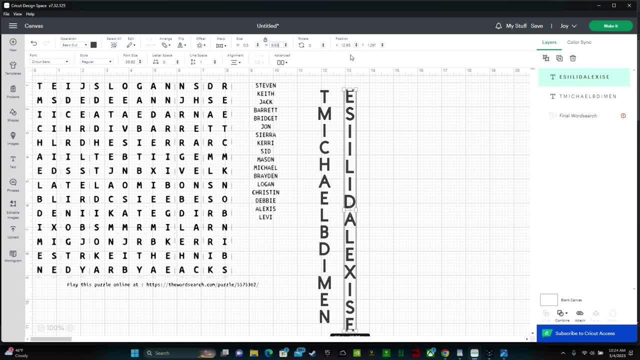 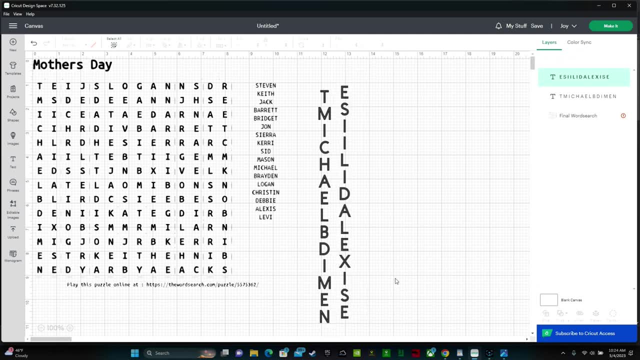 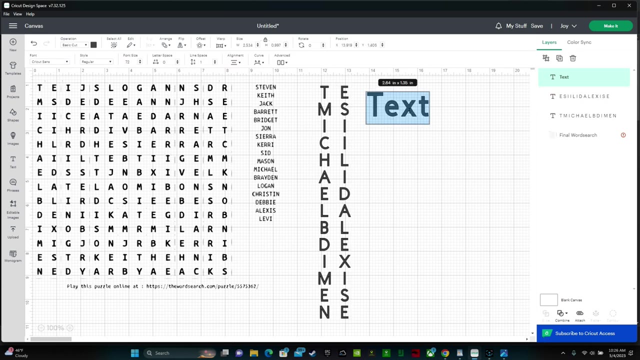 this one, 9.656, and let's say i put this one up a little higher and i want them to be aligned. i can highlight this whole thing and click align and then align it at the top. so now the letters should line up. we're going to repeat this process for the whole project. i'm not going to worry about. 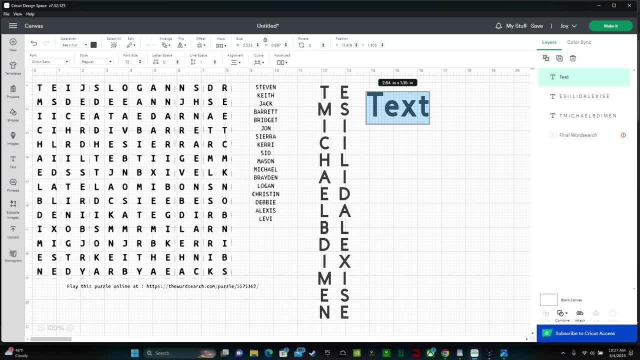 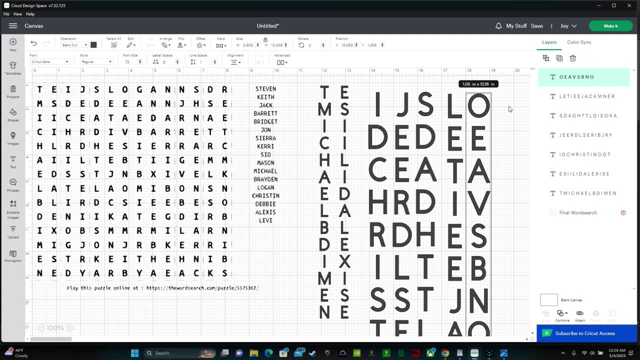 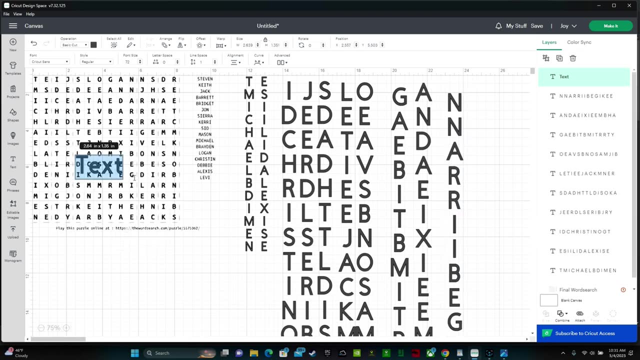 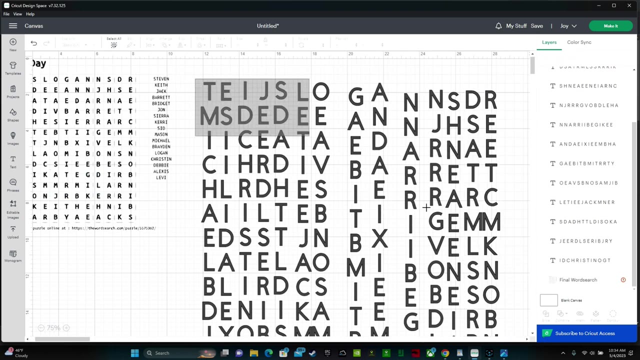 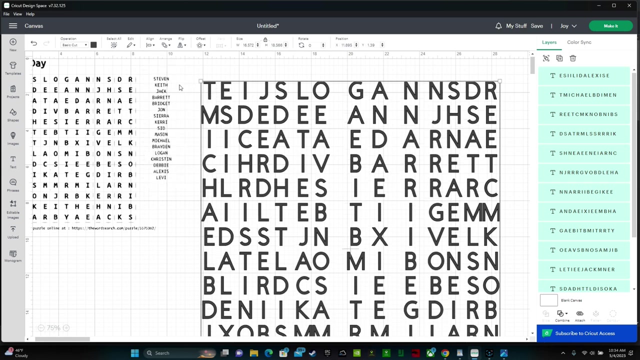 aligning any of these letters until the end. i just wanted to show you how to do it real quick. and then i'm going to highlight everything and click align- align it at the top. and then i'm going to click align and distribute horizontally, and now everything is aligned perfectly. 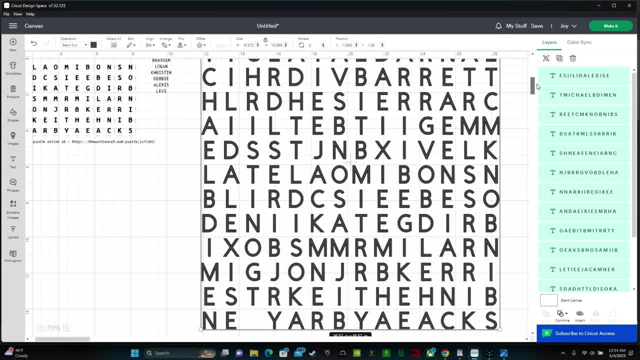 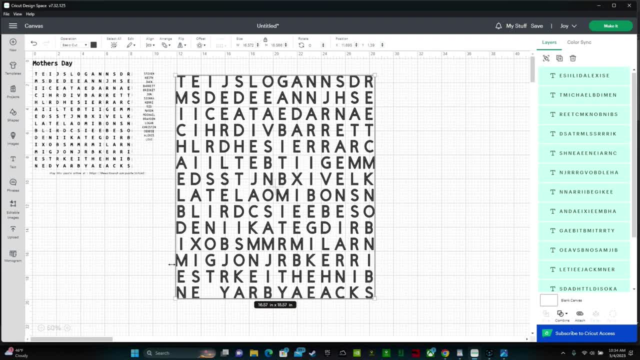 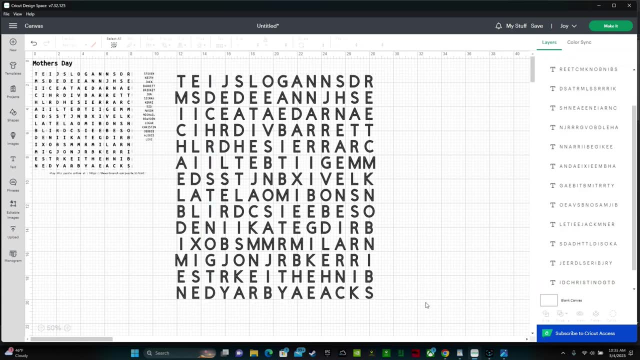 let me zoom out for you for a second. um, i missed one letter here. it says: and then i'm going to highlight everything and click align, and then i'm going to click align and distribute horizontally. it's a d. so now i can highlight this whole thing and resize it as needed. 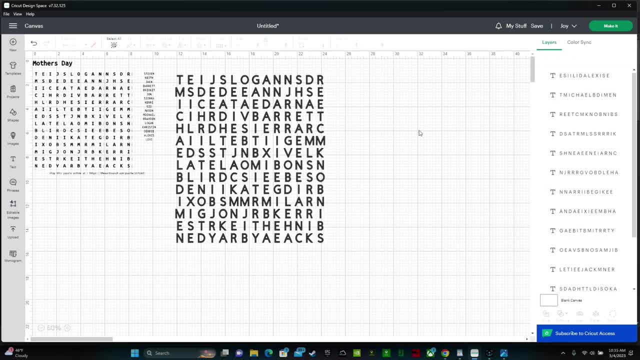 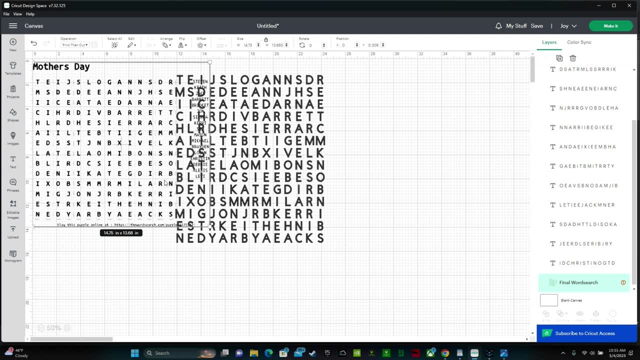 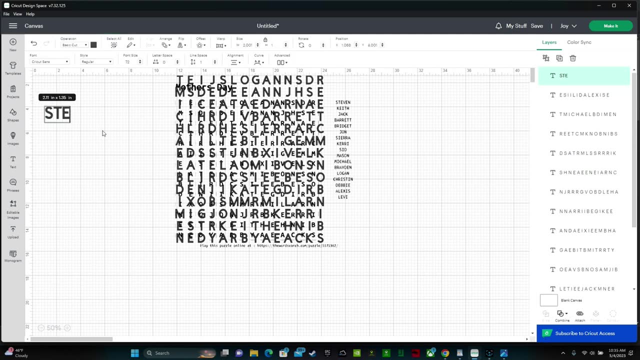 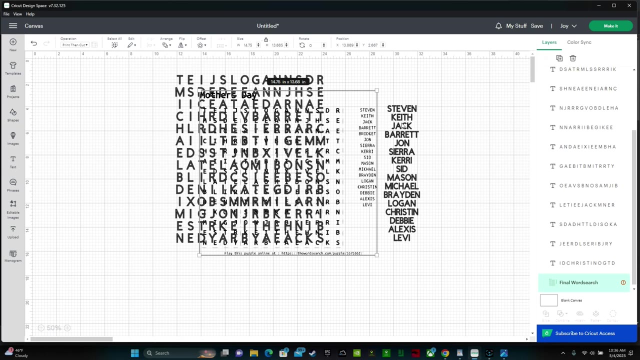 just highlight and shrink. next, i need to type out the names over here, so just like you see them here, i'm going to make this bigger so i can see it make a new text box. i'm going to write stephen, double check. all right, now i can delete this whole crossword. i don't need that anymore. 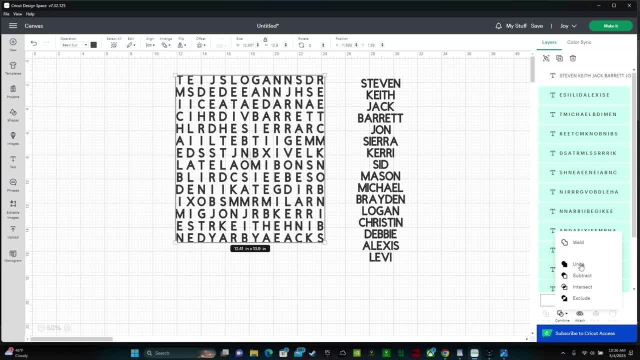 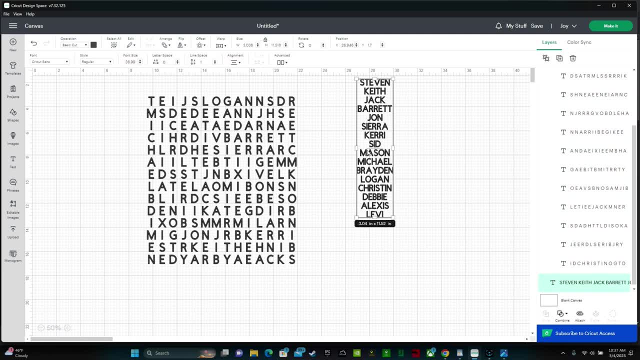 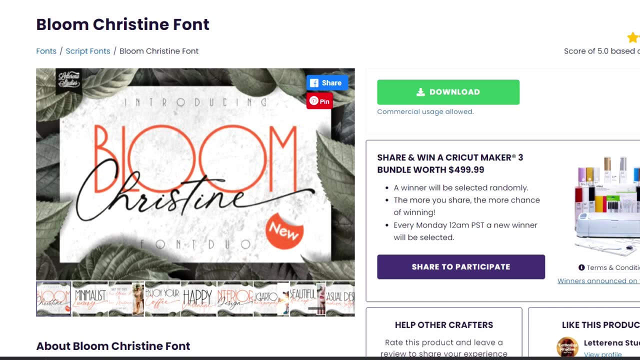 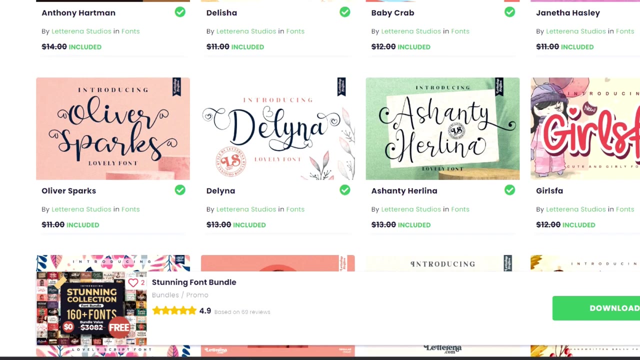 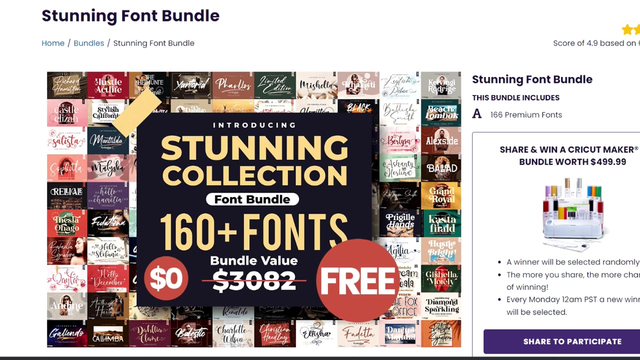 i'm going to highlight this and click, combine and unite, because i don't want them to go anywhere in this. i want to shrink down physics to the section here, so all the classes i want to create. now what you're going to want is a item box that i have and notice some of them are pretty flat and they do come up a little. 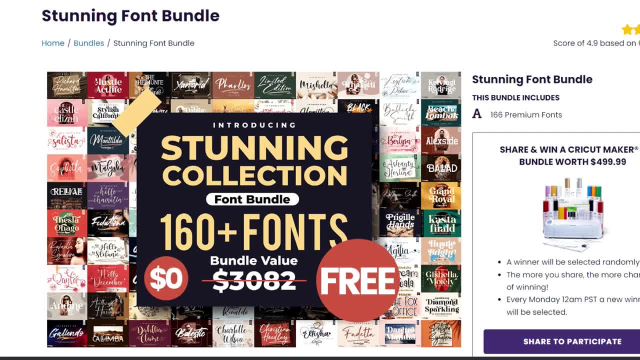 too easily, so i think i'm going to want to slide it down so that we have this piece of cake in this section, on this page right here. i'm gonna bring this down into the輔 only thing they're giving away for free. creative fabrica is running an incredible mother's day. 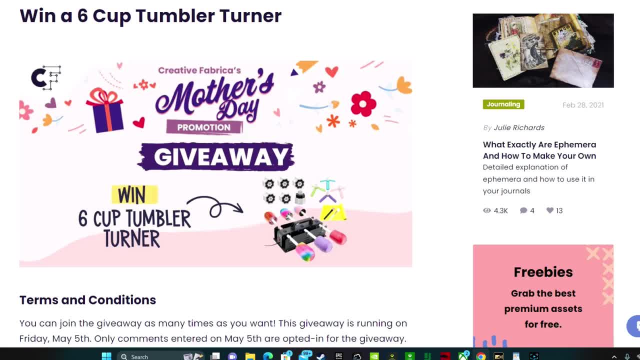 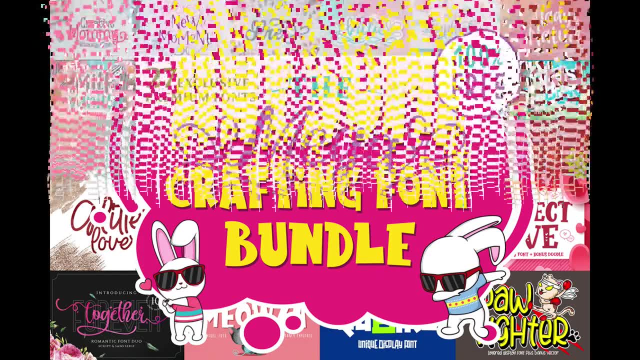 promo that includes free bundles and daily giveaways. that's a total of 14 free bundles. all of the bundles are free to download and includes so many great fonts and graphics to help you make the best cricut projects, just like the one we're making today, if you're not already. 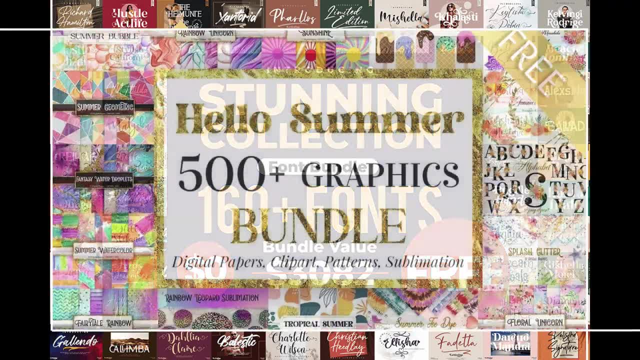 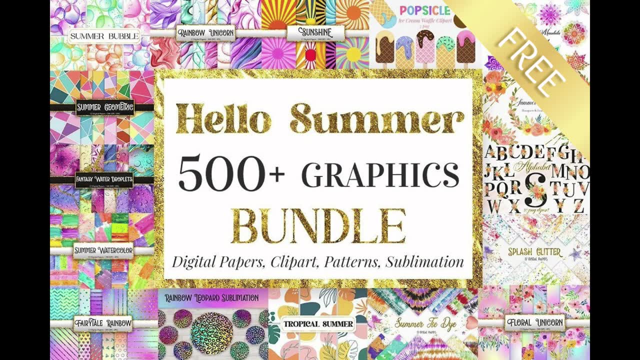 a subscriber of creative fabrica. you can try them out with their free trial offer. you can access millions of fonts and designs for free, and my favorite part is that a commercial license is included. this is the license that you need to sell your crafts legally, without fear of getting sued. 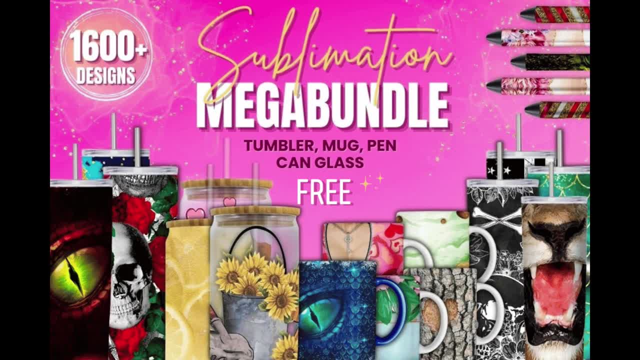 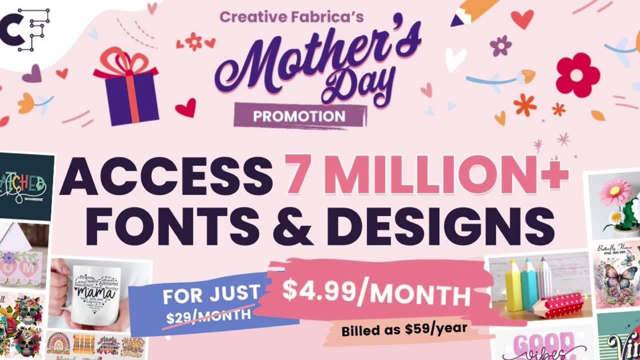 if you decide that you love creative fabrica as much as i do and want to subscribe to their yearly all-access subscription, you can sign up for just four dollars and 99 cents a month. this limited time promotion will save you hundreds a year over the regular 29 a month. 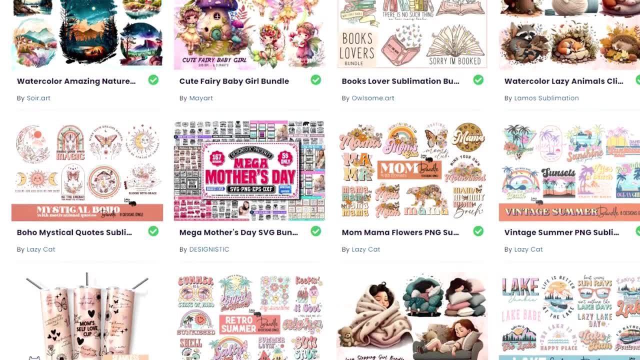 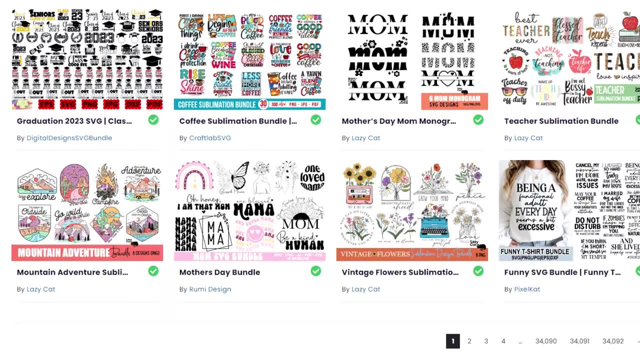 the all-access subscription gives you endless creative possibilities, and after you sign up for the free trial offer, you will also get tickets to over 7 million digital fonts, graphics, Creative Fabrica, Spark, creative online classes and so much more. To download this huge bundle, all you have to do is 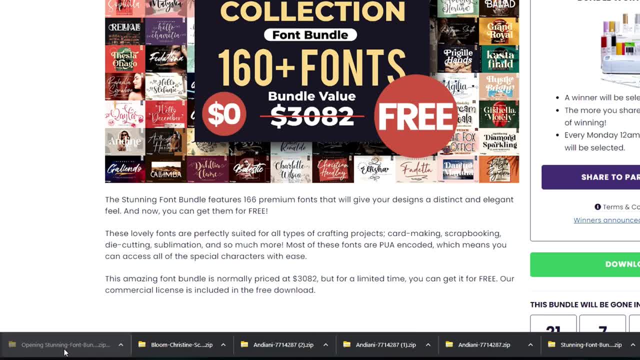 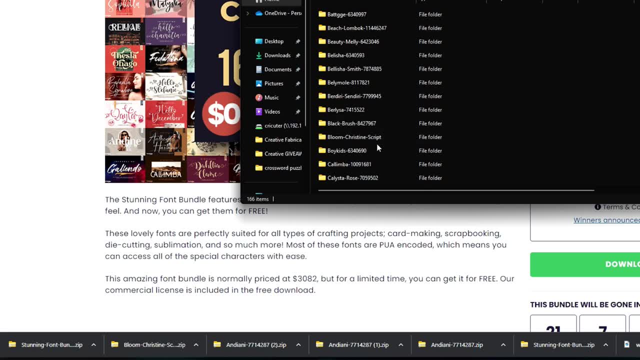 click download and it gives you a zip file full of all of these different fonts. So, like I said, the one that I'm using is called Bloom Christine font and it gives you two different types: There's Bloom Christine script or there's Bloom Christine sans serif. So I'm going to download both of them in the OTF files. 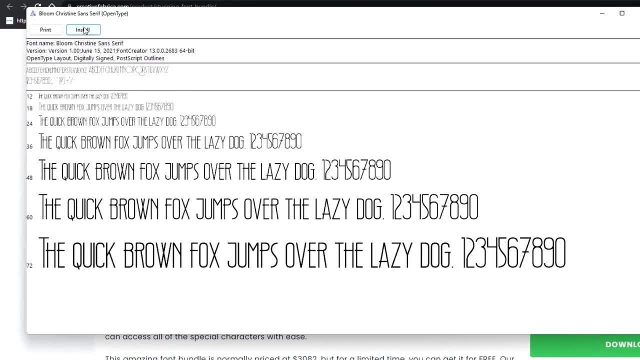 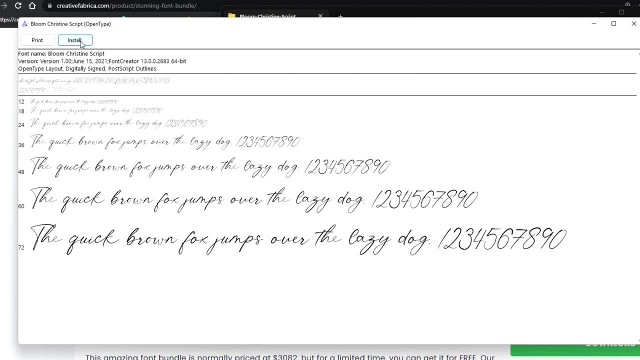 So you can double click it and just click install and repeat that same process for this one. Once you've installed your font, you need to go back over to Design Space and refresh the page. you need to go back over to Design Space and refresh the page. 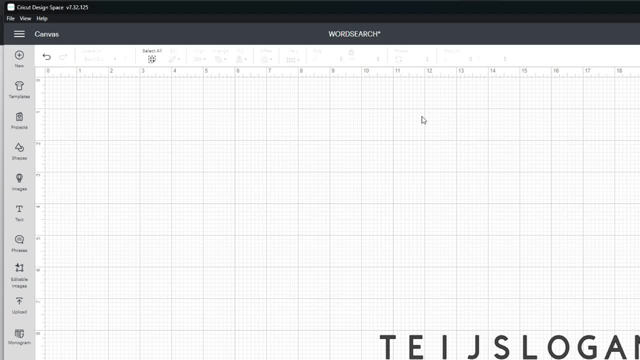 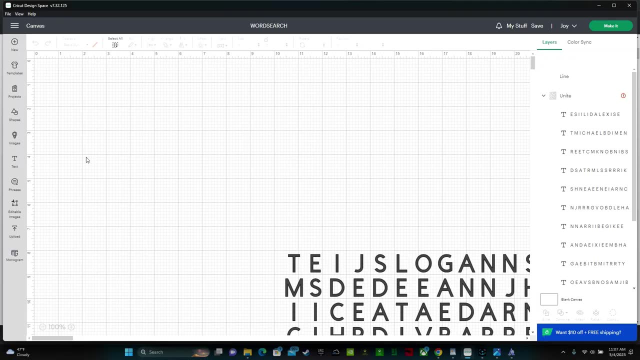 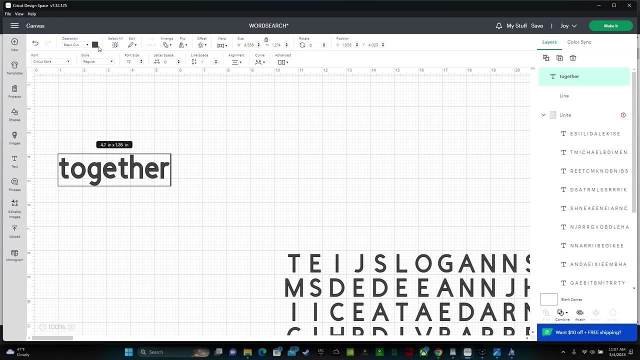 Make sure you have saved your project before refreshing the page. Then click view reload. The next thing that I'm going to do is type out the word together. So I'm going to click text and then type out together, and then I'm going to change the font to bloom. So you need to click system, because it's one. 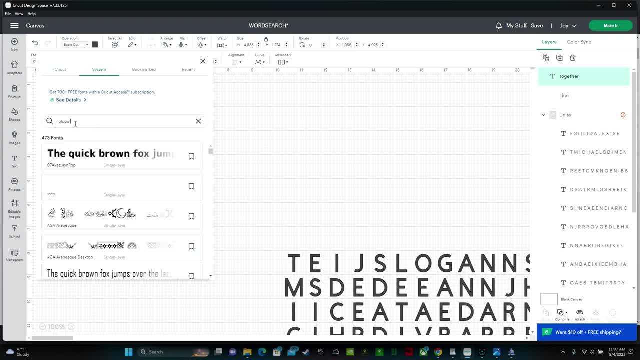 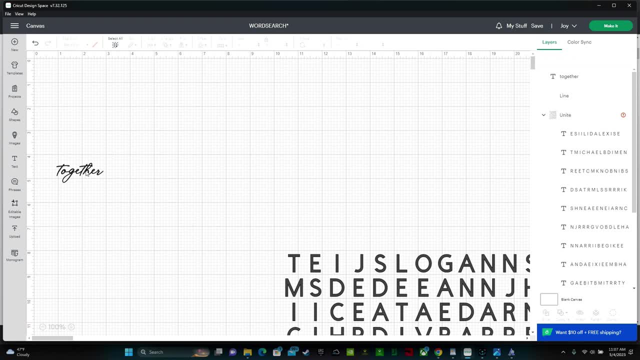 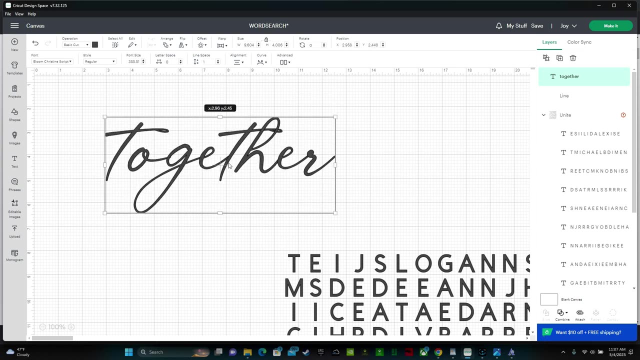 that we downloaded and search for bloom. I want to use the script, so select that and we can see together. but I'm not done yet. I want to use some special characters to make it look fancier and I want to make this T capital, So to access. 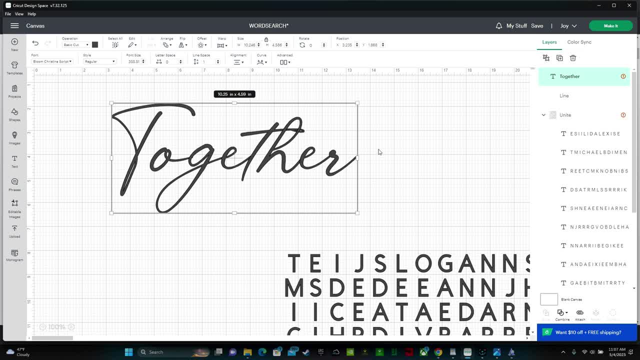 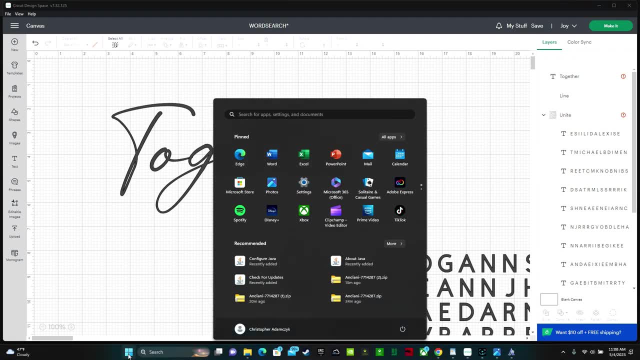 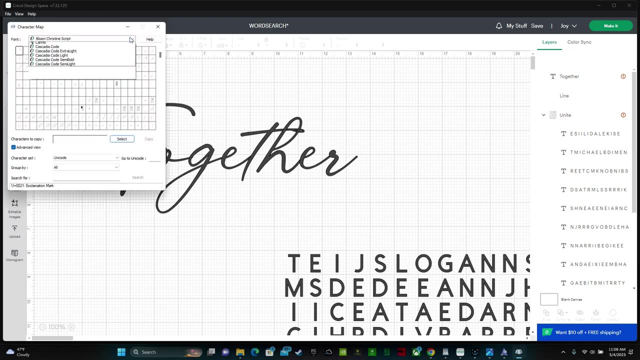 the special characters, we need to use something called a character map. I'm using a Windows computer, so what I do is go over to the start bar and type in character map, Select it. Then you want to search for the font, So I have bloom Christine script. 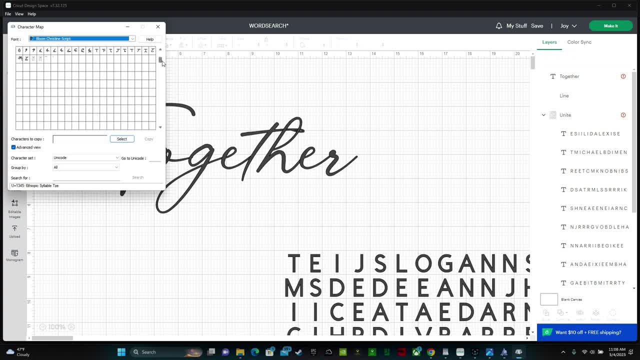 and here it shows you a bunch of the letters, but these aren't the ones that I'm looking for, So what I need to do is click group by and go to Unicode sub range, and then scroll to the bottom of this one and select private use. 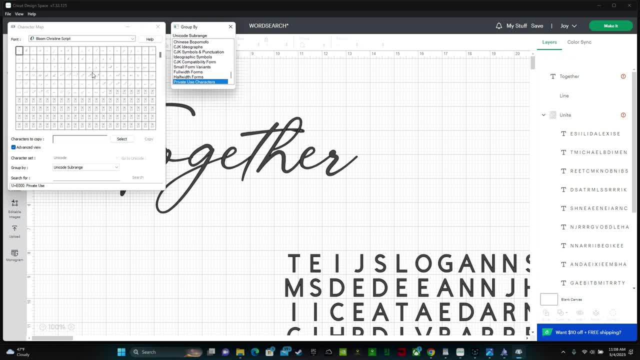 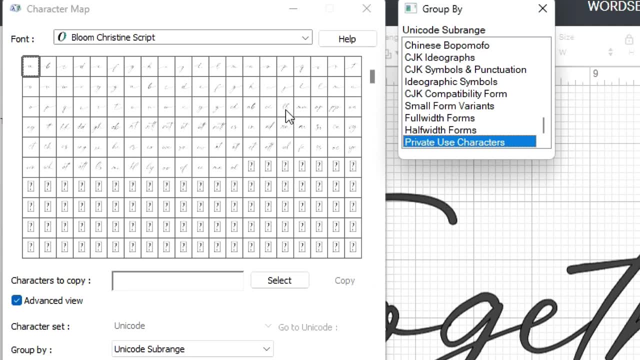 characters. Now you can see we have all of these really fancy letters. It's a little difficult because they make them super small and hard to see, but you can click on it and it will make it bigger. So I'm trying to find the letter R, which I 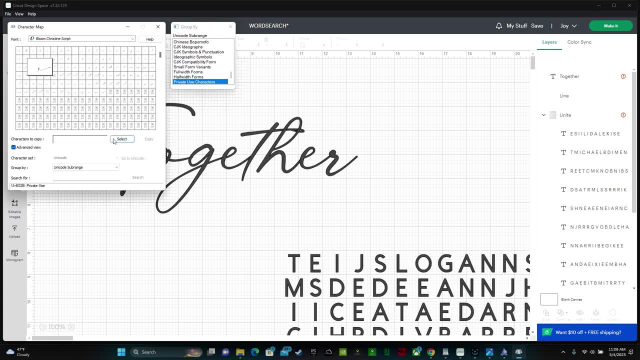 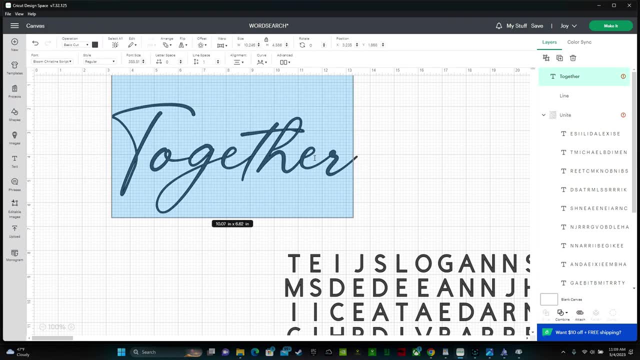 think is right here, so that I can click, select and copy. Now, if I go back to here, I'm going to delete this R and do control V to paste, And that gives us a really pretty R. Now, below this, I want to write: we make a. 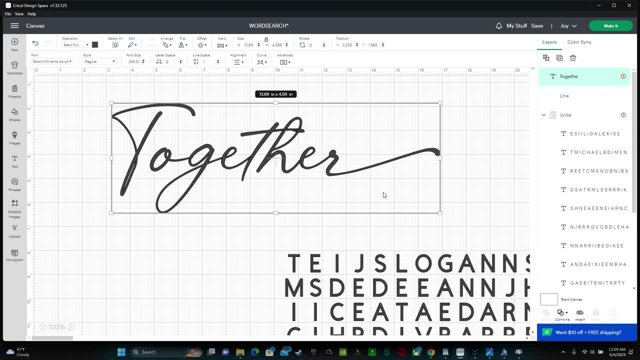 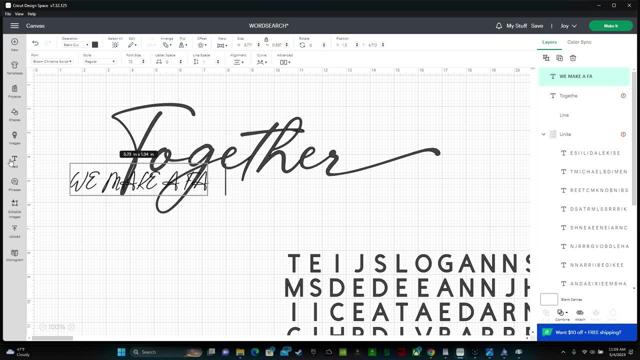 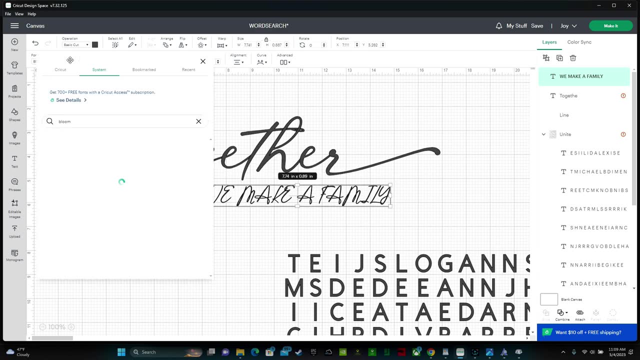 family, but I want it to be in more of a classic font. So I'm going to click text and type in in all capitals: we make a family. but I'm going to change this font. This bloom one has a plain font, so let's see what that one looks like: a Sanson. 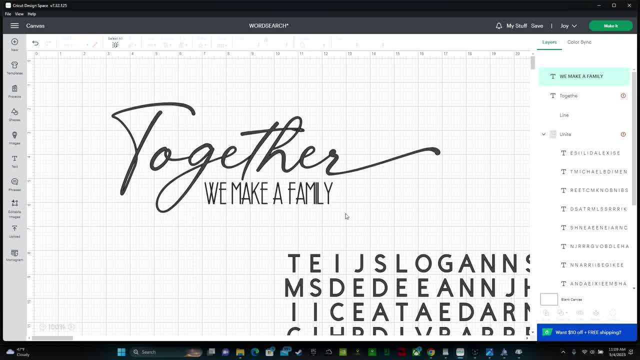 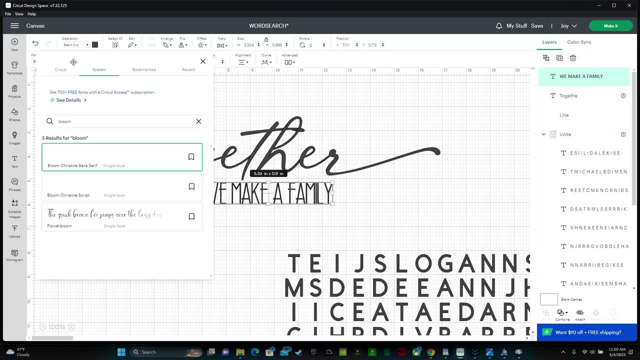 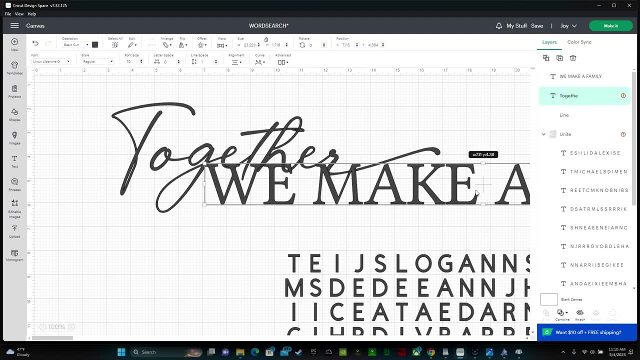 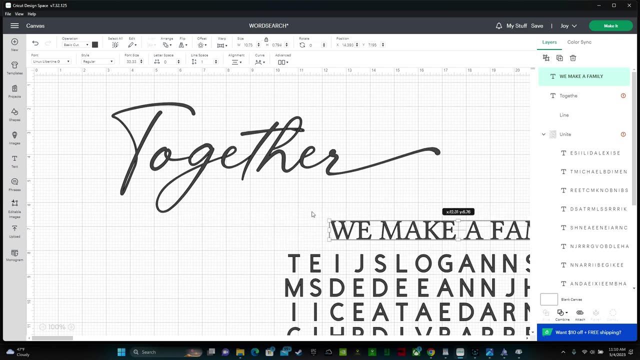 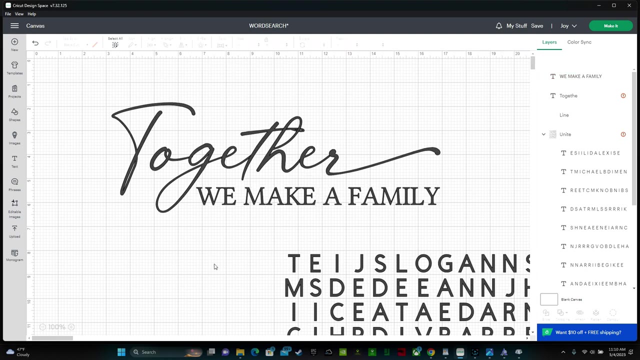 I don't like how that looks, so I'm going to find a different one. This font is called linex libertine G. I use this one all, So that's why it's called linex libertine g. I use this one all the time. I think I might have got this one from defontcom, so that looks amazing. So now I can zoom out, I can now change changes to the person better, and we're pretty good with this. Yep, Yep. Ok, So this is the one that I use the most among all of these options. Yeah, Cheers, Cheers. 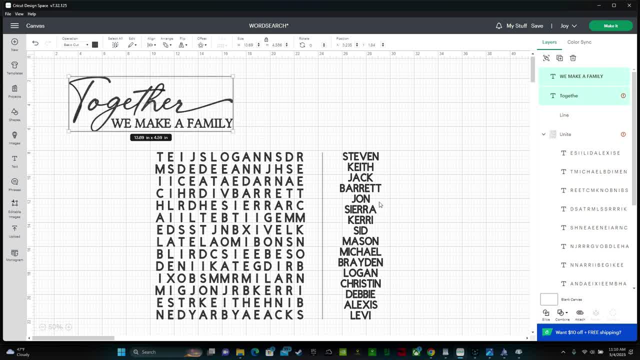 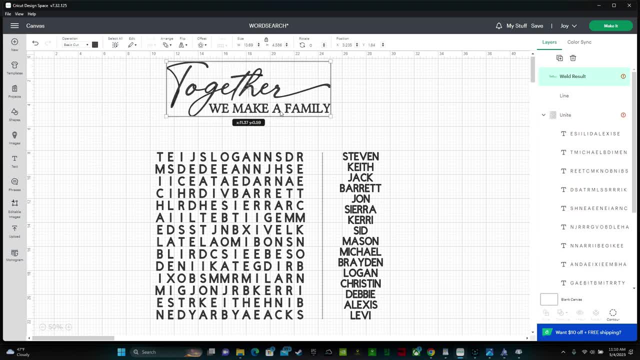 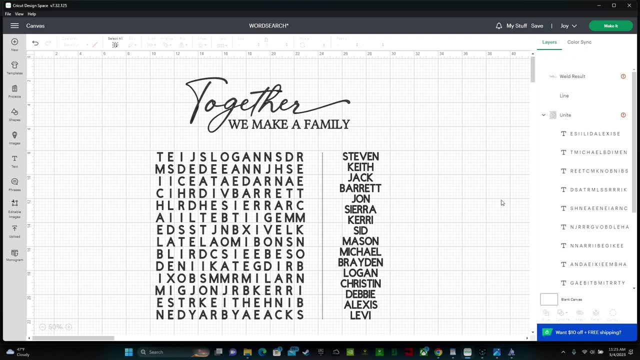 Cheers, Cheers, and I'm just gonna weld this together because I love how it looks and move this over. now I need to figure out what to resize this to. so I took a ruler and I measured my dry erase board and it's gonna be about 14 inches wide by 10. 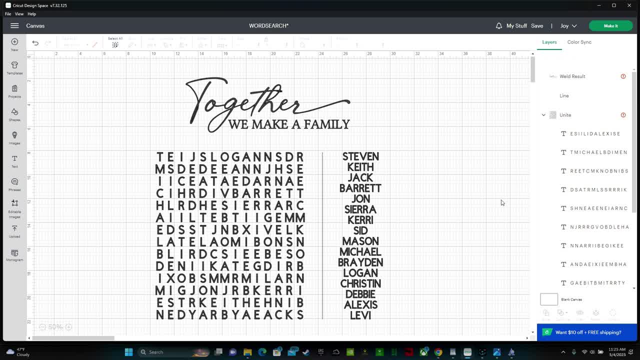 inches high. so I'm gonna go over to shapes and make a rectangle with those dimensions. I'm gonna use this rectangle as a template and delete it later, but for now it will help me figure out how big to make everything and where to place it. so click shapes. so click this unlock button and change it to 14 wide. 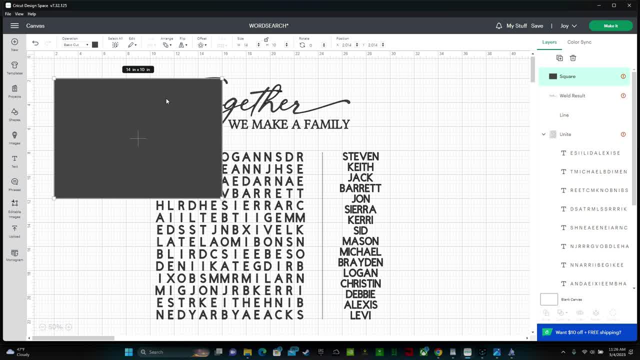 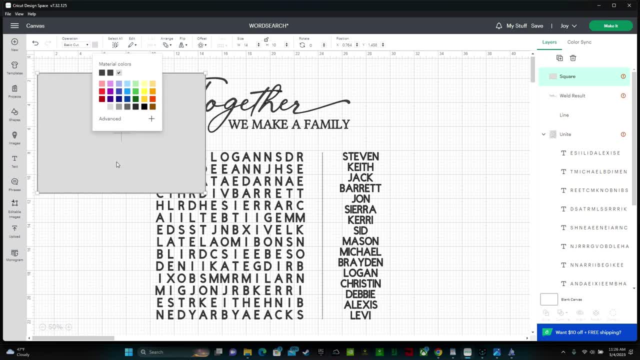 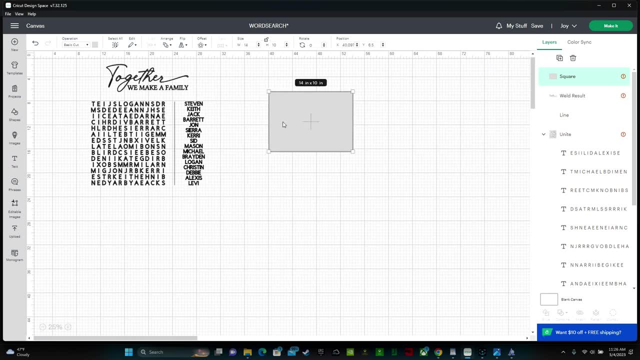 and 10 inches high, then I'm going to change the color to something lighter, like a light shade of gray, and I have to zoom out some more. now we have to shrink this down so it fits within this box. so highlight the whole thing and we're gonna start shrinking. 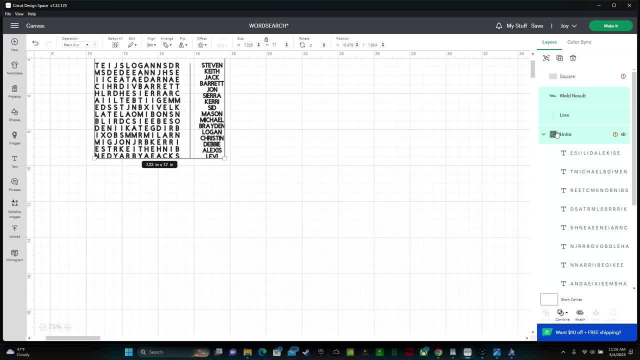 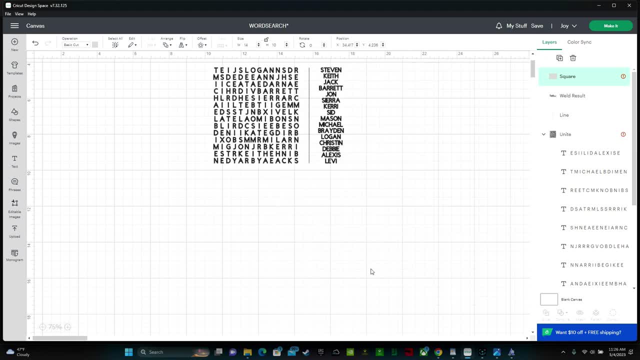 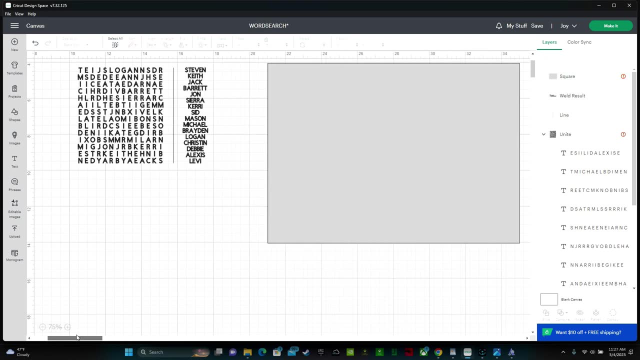 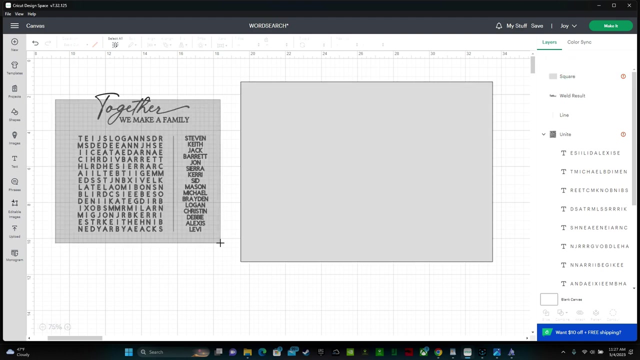 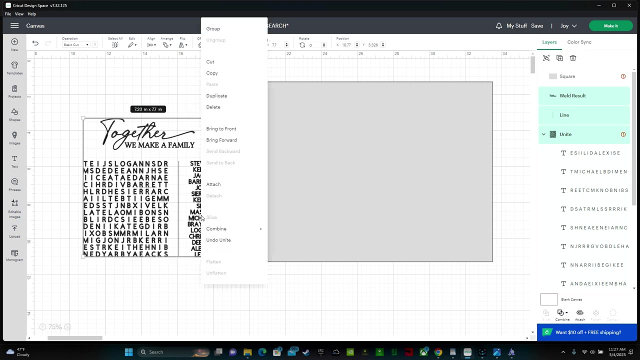 now I can zoom in and I lost my square, so click that and move it over. okay, I'm gonna take this and drag it onto here right now, showing up behind, though, and I want it to be in front so we can right click and click: bring to. 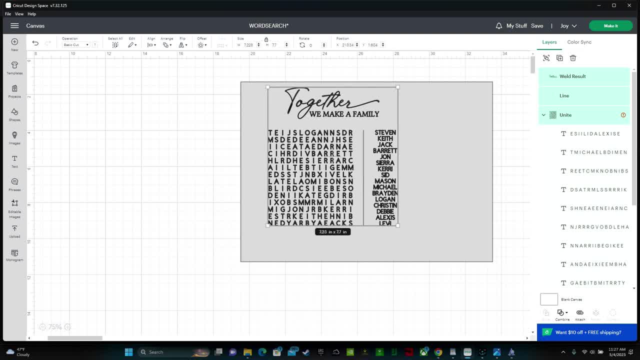 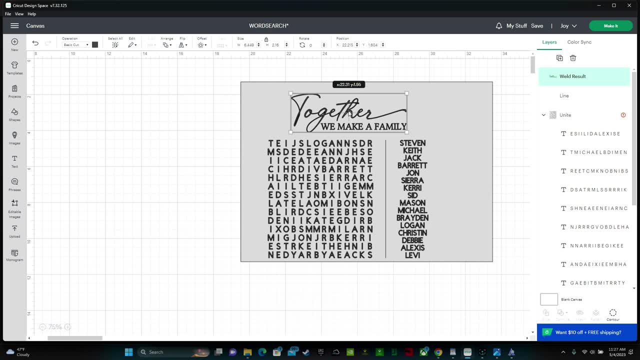 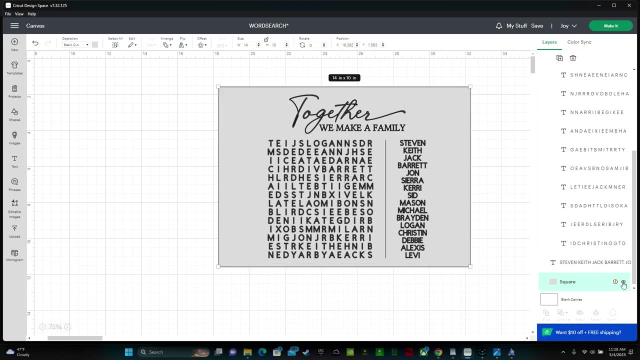 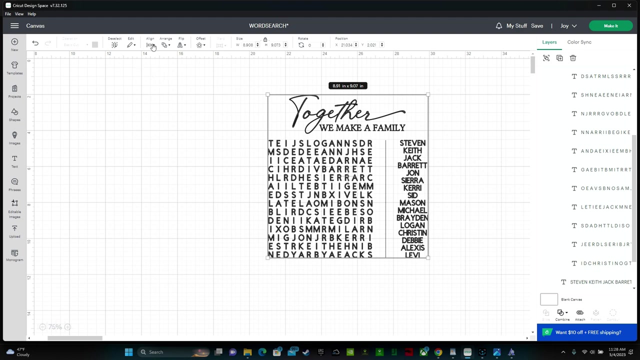 front. now I can enlarge it. I'm gonna take this and move it down. I'm gonna hide my rectangle for a second with this I tool and I want to attach all of this together, and then I want to Center this with this so I can highlight it, click, align and then center horizontally. now I can highlight all of. 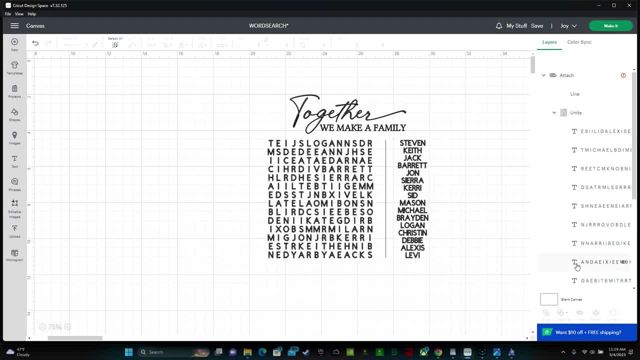 this together and then move it down to this point over here and then click here, and then click here, and then move it down, and then move it down to the and click, combine and unite. right now it's telling me that the size is too small. that's because this is still set to my Cricut joy. I have a couple. 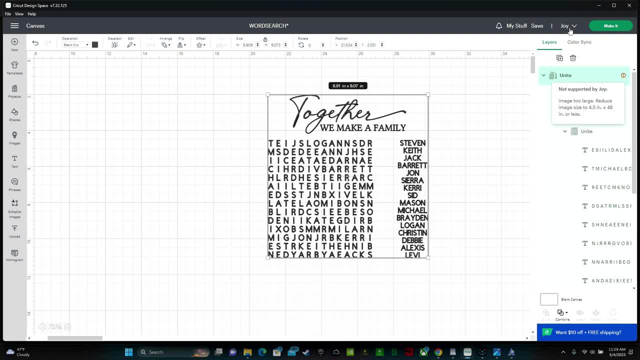 different machines. the last machine I used was the joy. so to change a machine, you just go up here and then change it to whatever machine you're gonna use. I'm gonna be using the Cricut maker and now I'm going to enlarge it to fit inside. 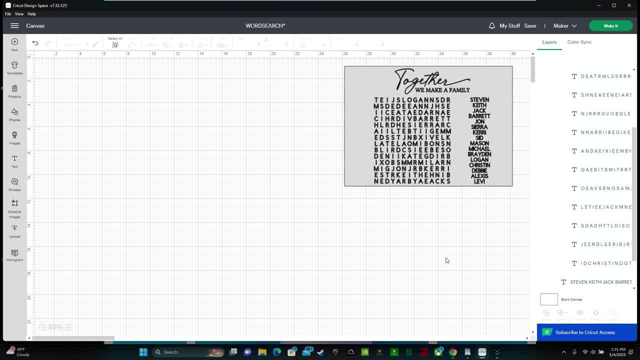 this gray box. now I am pretty much ready to make it. I think it looks good where everything is. so I want to take this gray box and delete it, or you can use the eye tool to hide it and then I can go to make it. everything looks good. 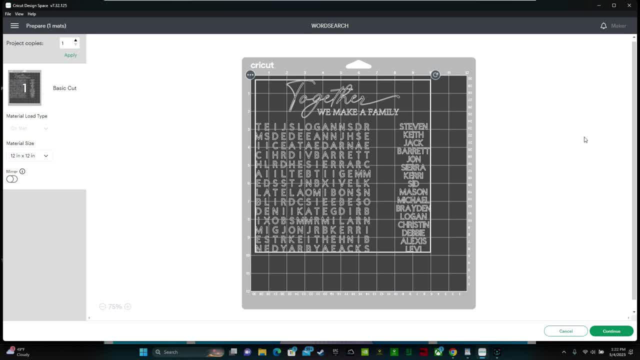 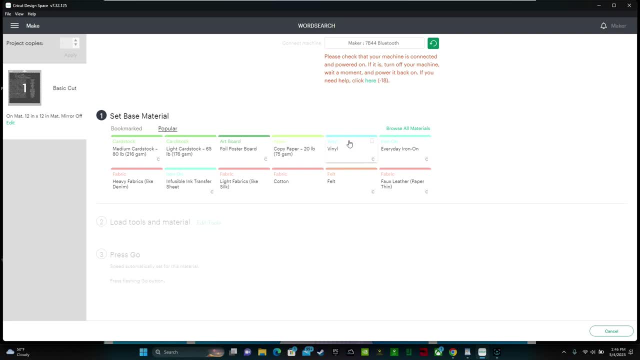 here. I don't need to mirror the image because it's not a heat transfer vinyl, so I can go ahead and click continue. the next thing you want to do is select your material. I'm using vinyl. I like to look at the image and then I'm going to go ahead and select the material. 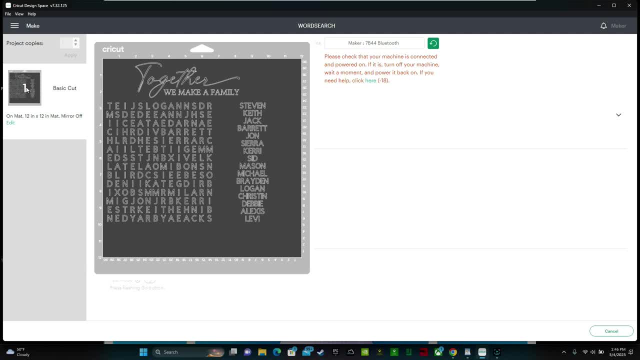 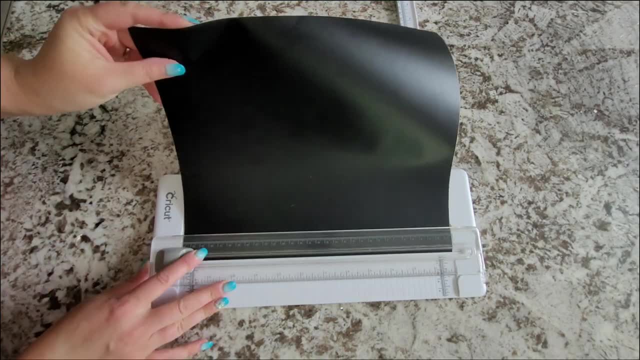 I'm going to look at my mat to see how big I need to cut my vinyl. I can see I need to cut it about 10 inches. now we can stick this to our mat. you want to take your sheet of vinyl and place it in the upper left hand corner of your 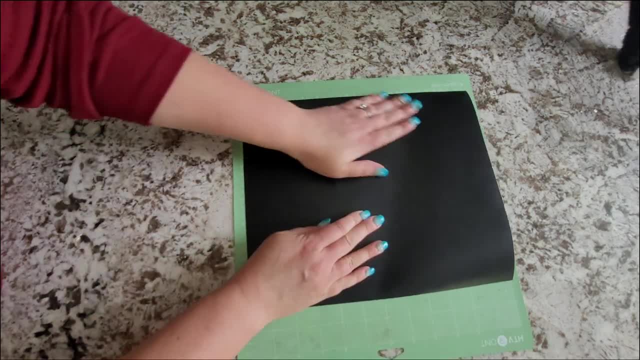 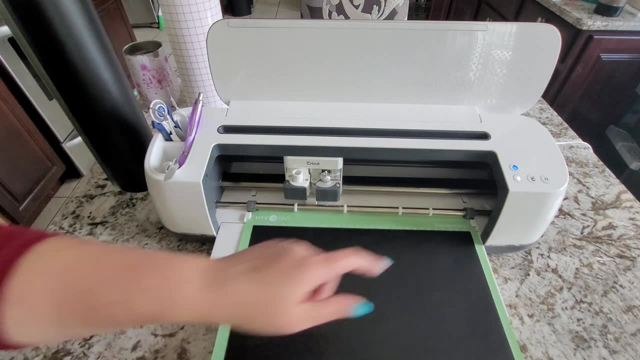 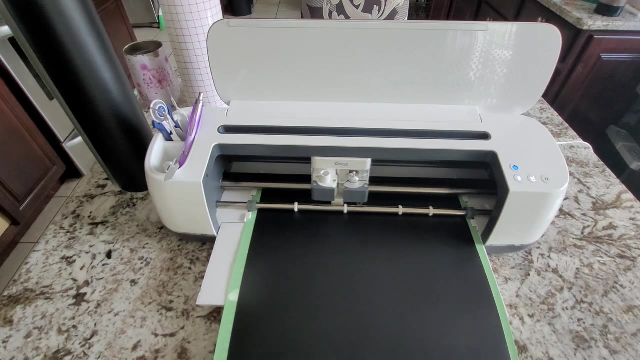 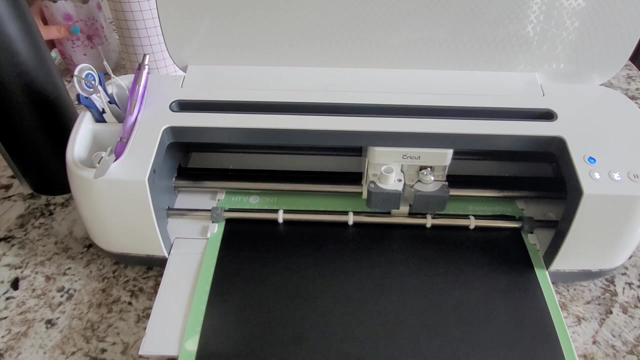 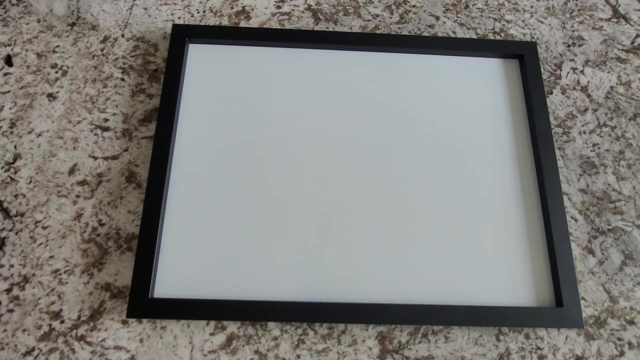 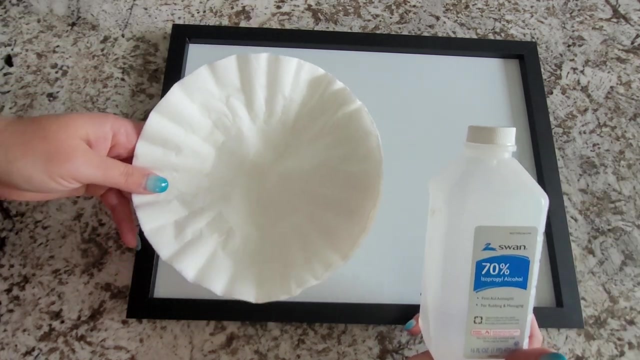 Cricut mat. I'm using a standard grit mat which is perfect for working with vinyl. next, you just have to load it into your Cricut machine. before you can apply your vinyl to your dry erase board, you need to clean the surface. I always clean the surfaces of my projects with isopropyl alcohol in a 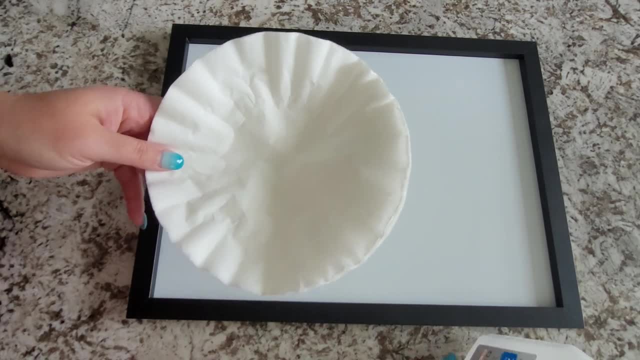 lint-free wipe, also known as a coffee filter. coffee filter is a filter that is used to clean the surface of your coffee filter. coffee filter is a filter that is used to clean the surface of your coffee filter. coffee filters are lint-free and they won't leave any residue on your surface. 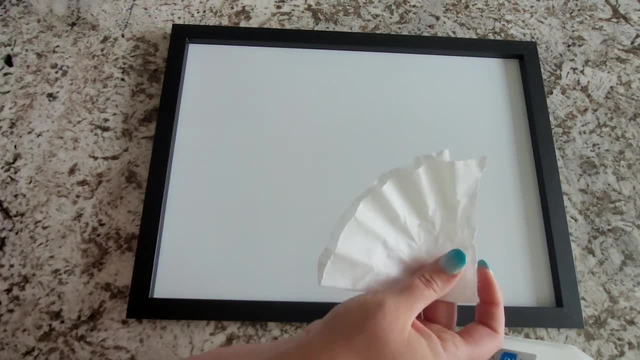 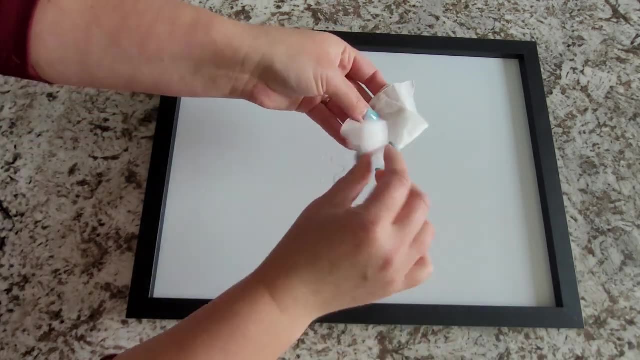 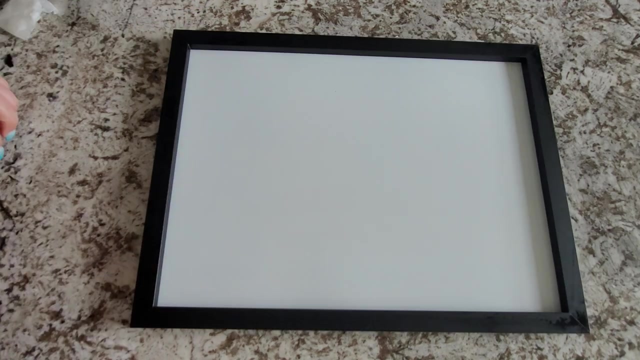 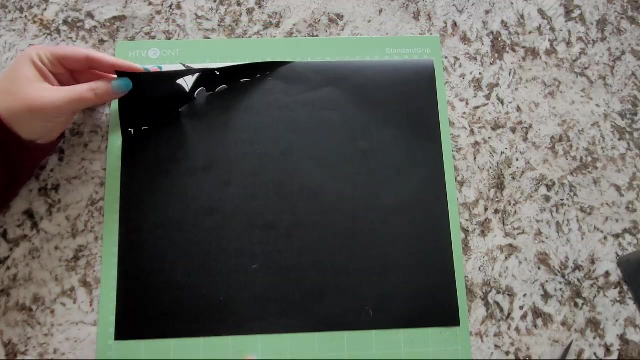 if you don't want a waste material, you could actually rip this up, because you only need a small amount. so pour some alcohol on your coffee filter and then rub it in. then we can put that aside and wait for it to dry while our machine cuts, and then we weed our project. 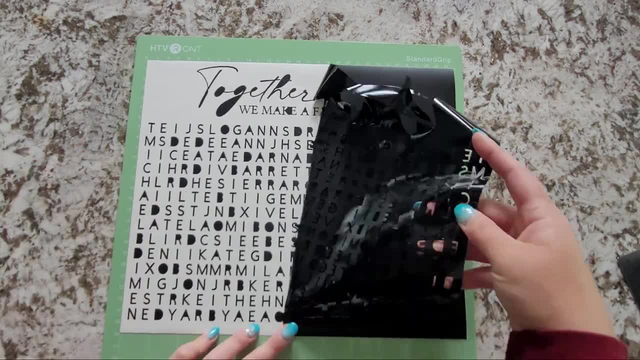 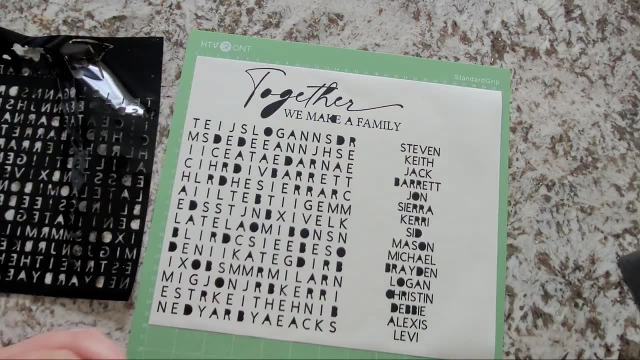 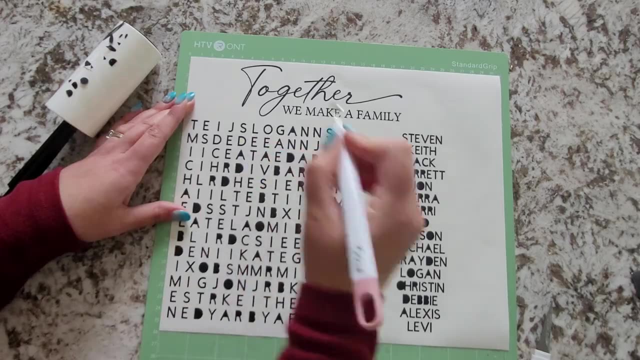 so this is our final result and I'm going to take our paper and sign it and we're going to get the paper out. so I'm going to go ahead and just hold this up and we're going to take it out and we're going to start by taking out of our coffee filter and just wipe it right. 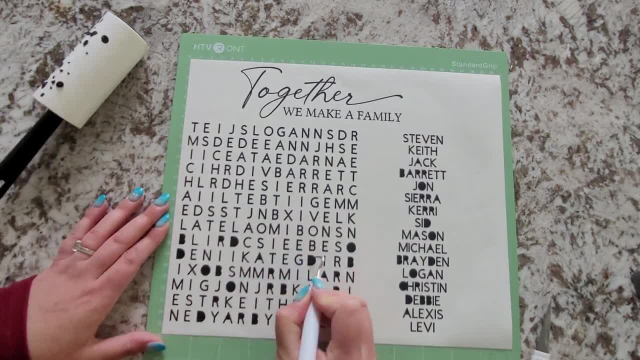 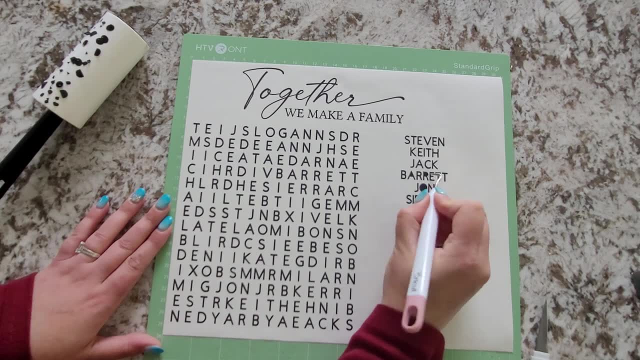 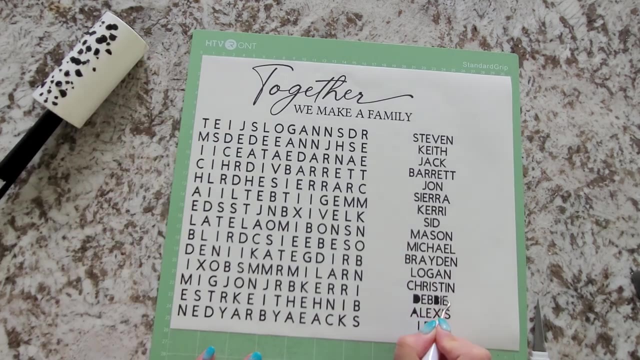 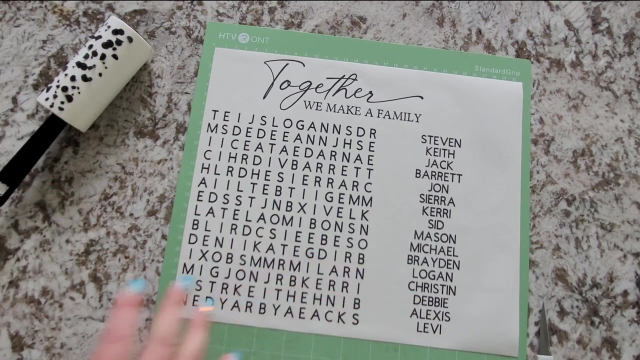 on the bottom of our machine. I'm just using my clean cotton cloth and then I'm going to wipe it off with some alcohol. so I'm just going to wipe it off and then I'm. now we need to use our transfer tape to transfer it from here to the dry erase board and, if you, 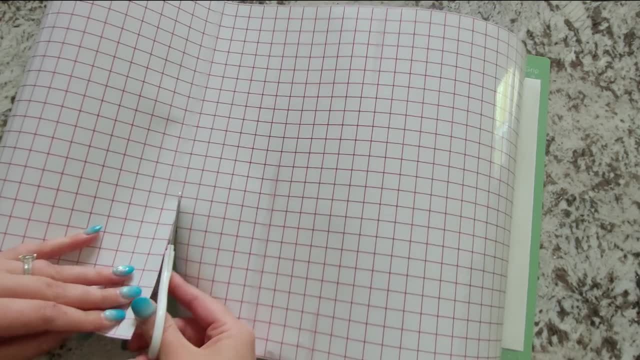 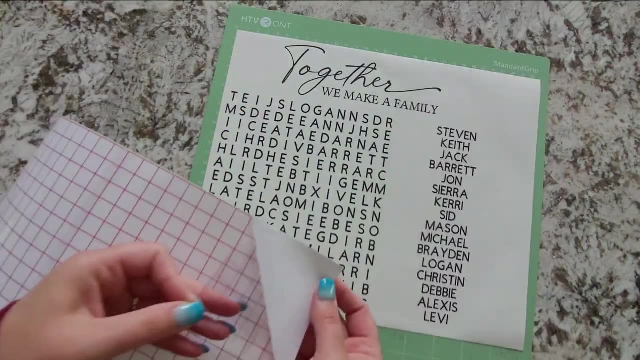 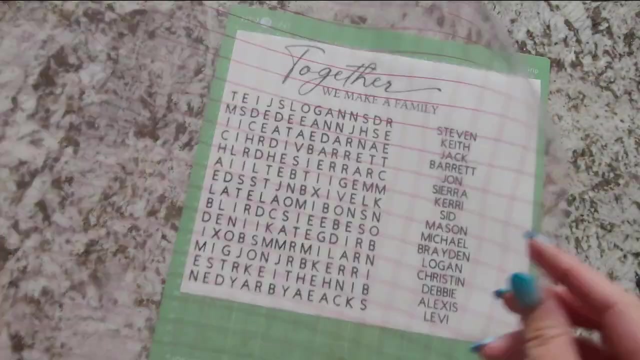 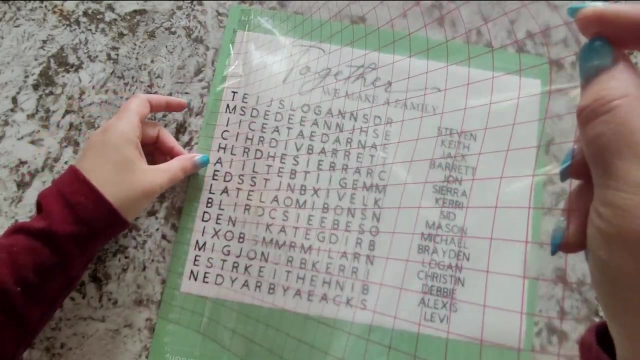 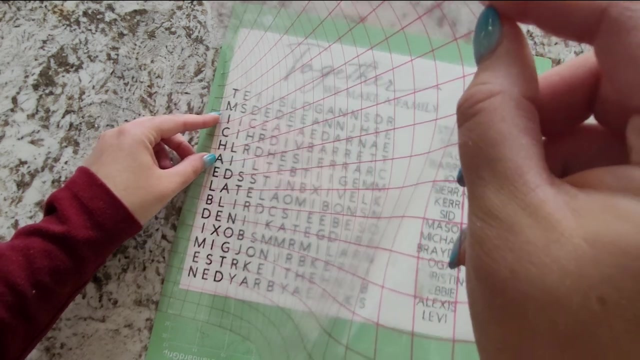 didn't know this already. transfer tape is reusable, so you can reuse the sheet over and over again. peel the transfer tape from the backing and then carefully line it up. I'm gonna go left to right. you can also use the grid lines on this transfer tape to help you get it in the right spot. 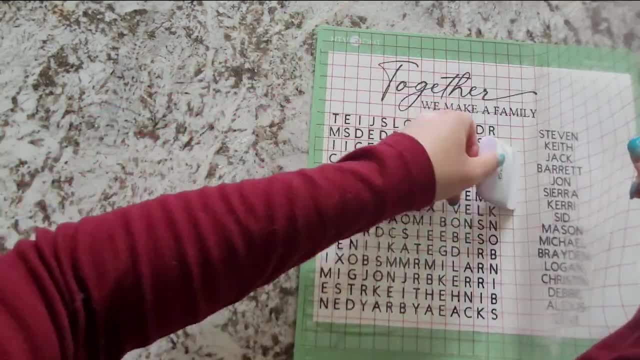 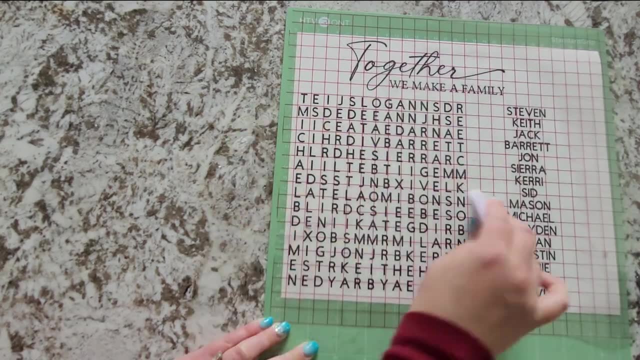 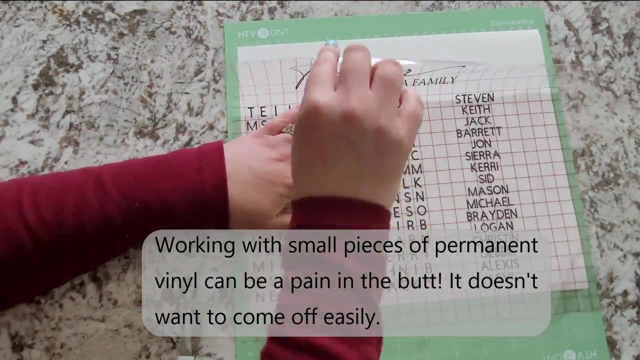 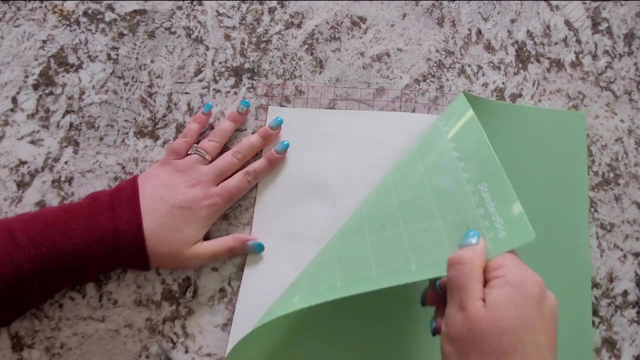 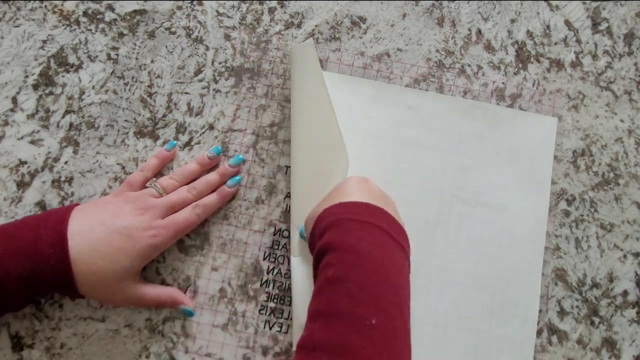 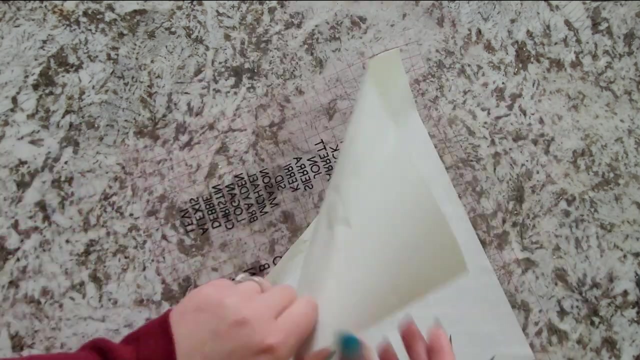 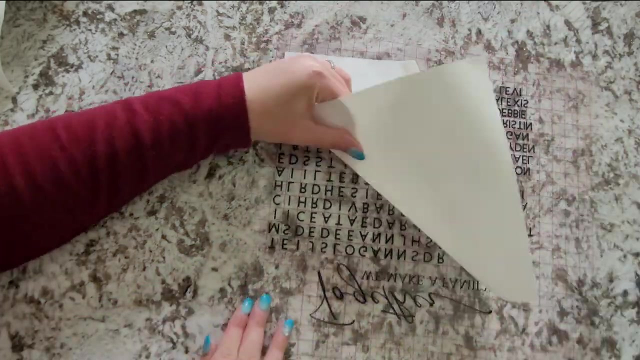 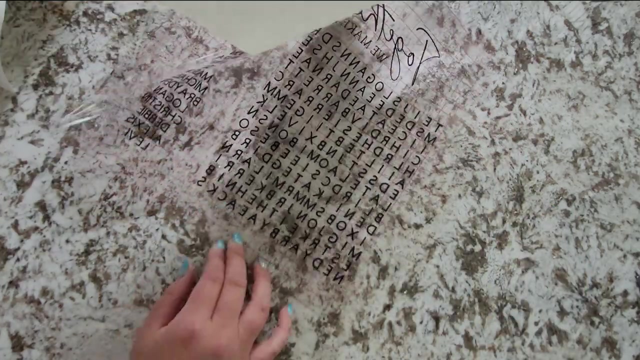 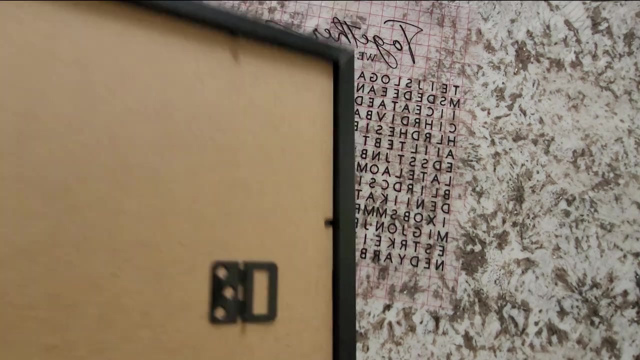 I think it might have some better luck if I peel it from the back. ah, we did it all. right now we have to transfer it to the dry erase board. I want you to flip over your dry erase board and remove thebands at the top so that you can sort of see them together. 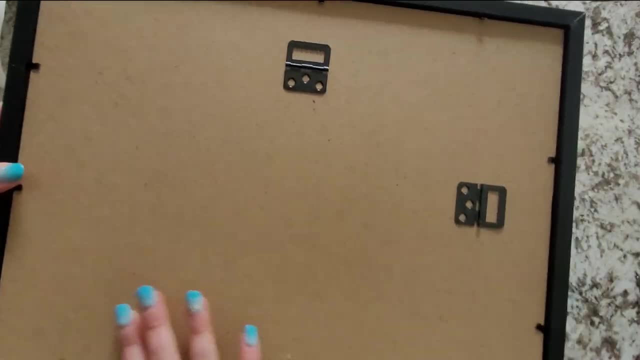 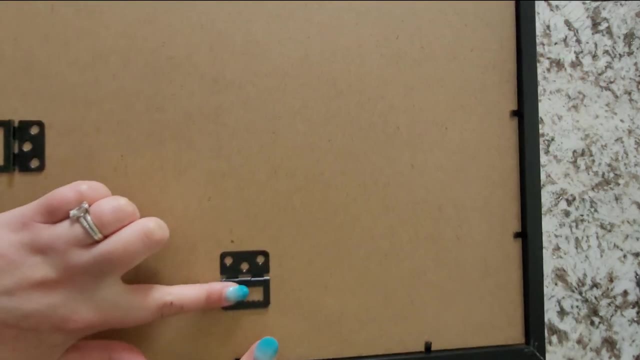 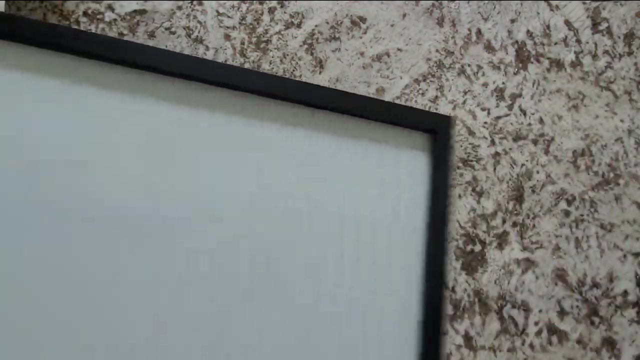 erase board and pay attention to where the mounting brackets are, because you don't want to stick your vinyl on with the mounting bracket, like on the bottom. so make sure your mounting bracket is on the top and then move this aside. now comes the part where I hold my breath and 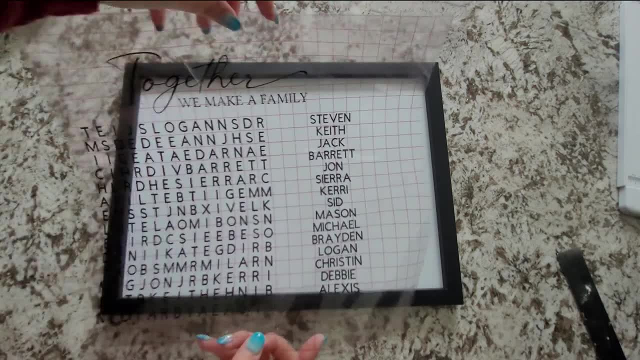 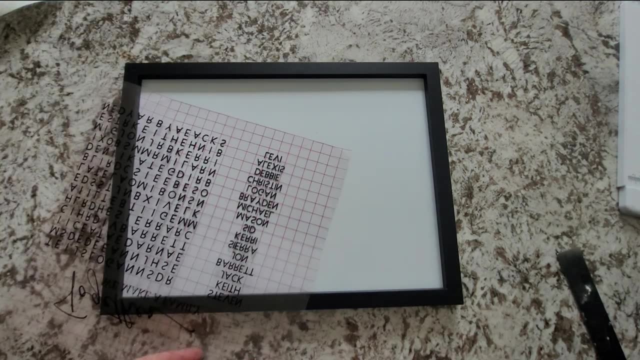 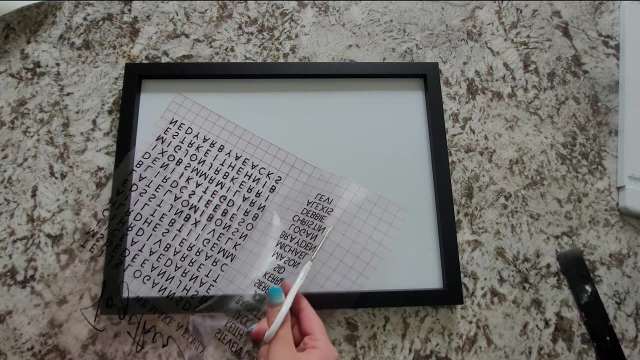 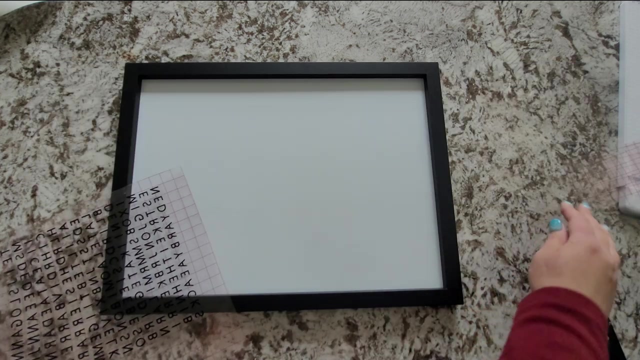 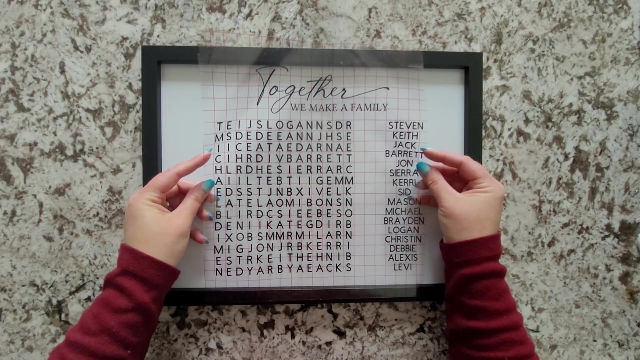 I'm going to cut off this extra strip just to make it a little bit easier for myself. I feel like when there's less sticky stuff hanging out to get stuck on things, it's easier. so I'm actually using my gridlock lines right now. there's a line right on the bottom of the frame that lines up. 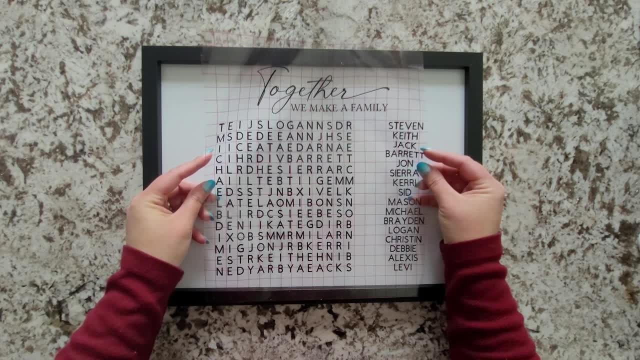 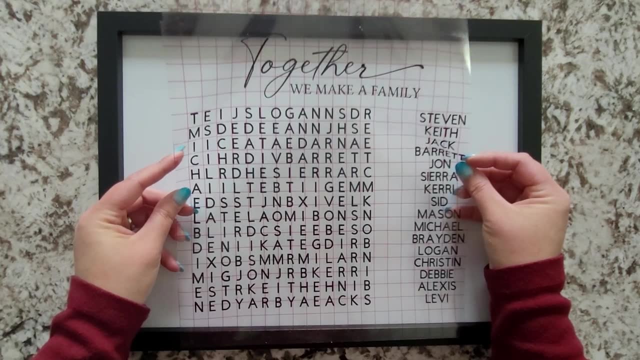 perfectly. so I'm lining up the bottom line of the transfer tape with the frame to make sure it's straight and I'm just kind of eyeballing where it looks Center. now I'm placing the vinyl down right in the center and I'm gonna work my way to. 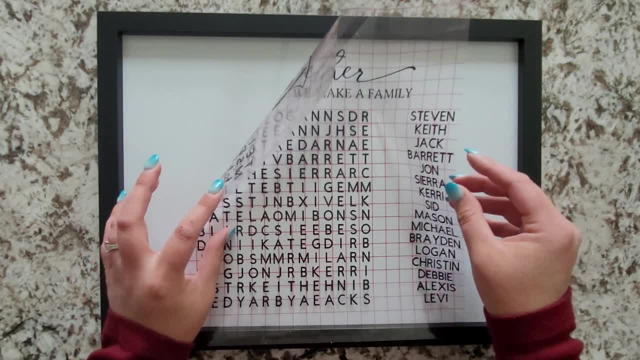 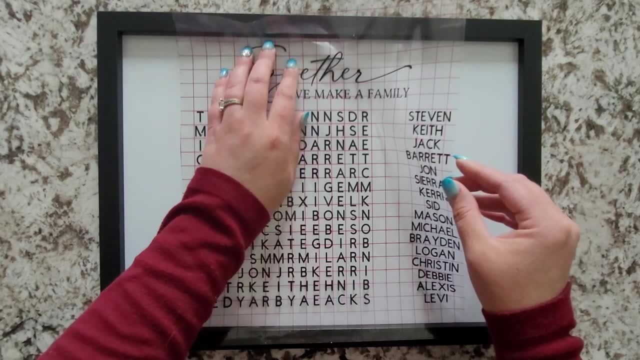 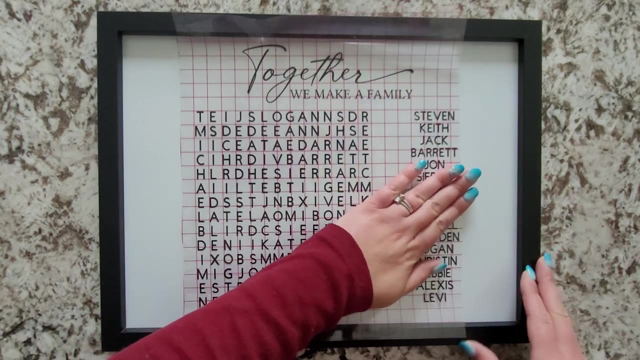 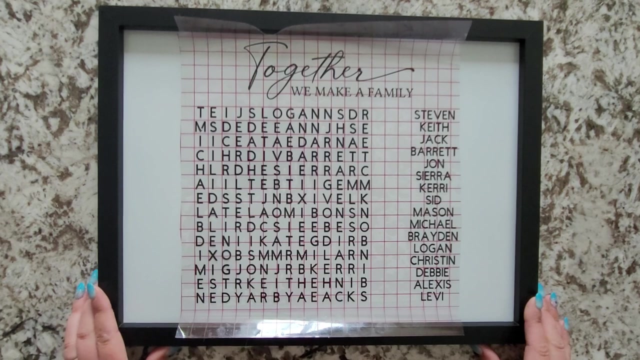 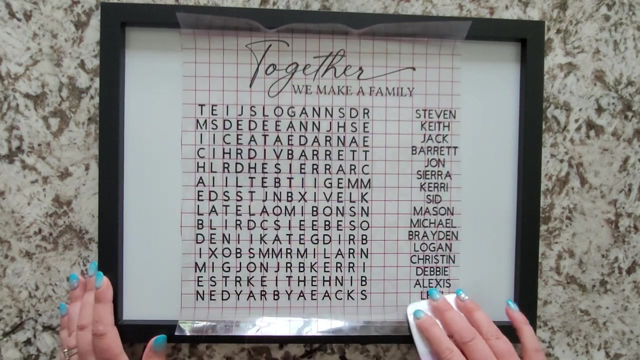 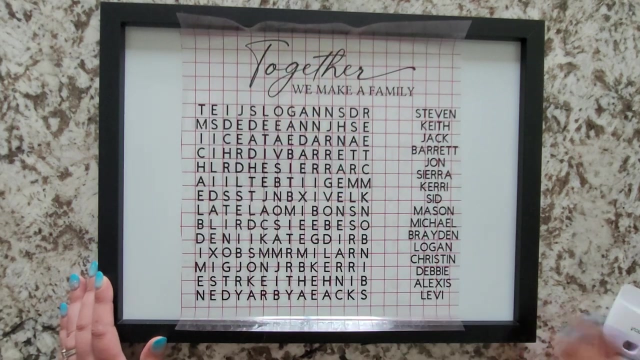 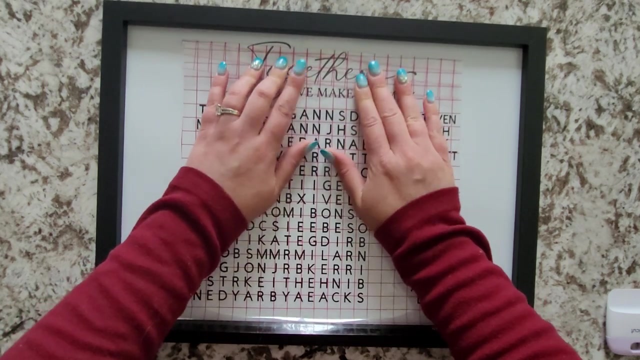 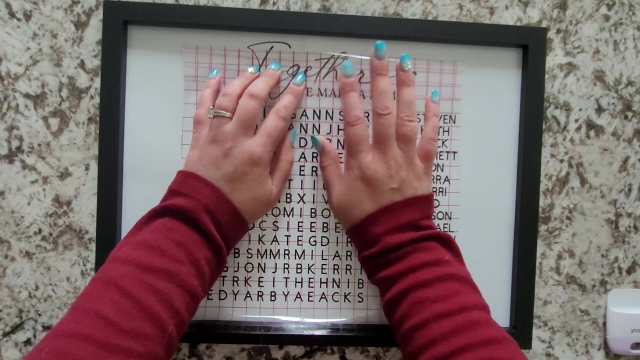 the outside ever so carefully. whoo, now I can breathe. all right, take your scraper tool, smooth it down nice and flat all over, and then we can peel back the transfer tape. so I don't pull straight up, I fold it all the way flat back, so it's facing my body and flat on the dry erase board. 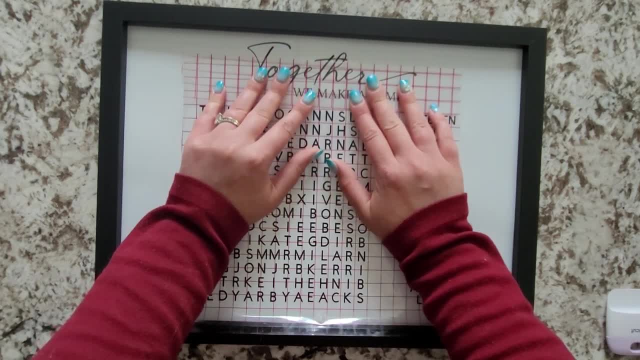 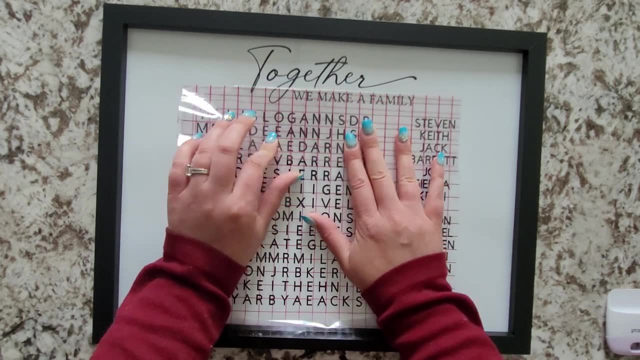 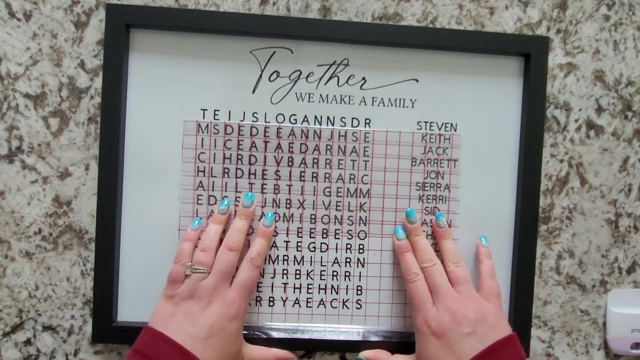 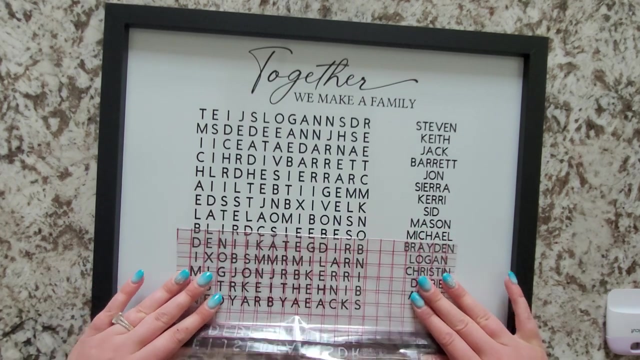 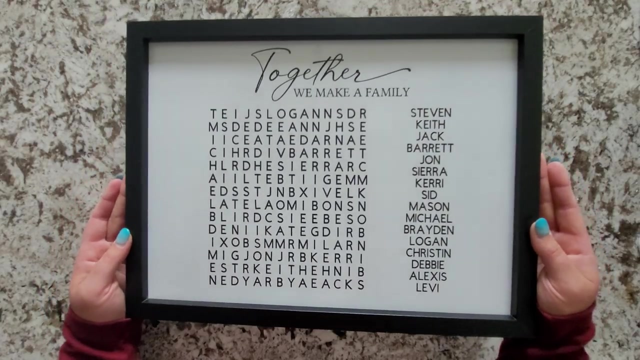 and then I slowly pull it towards myself. you- sometimes it helps to wiggle a little bit side by side, so I'll pull down on my right hand and then I'll pull down on my left hand and just slowly wiggle my way down, so you guys are never gonna believe what I did. I'm sitting here looking at all the 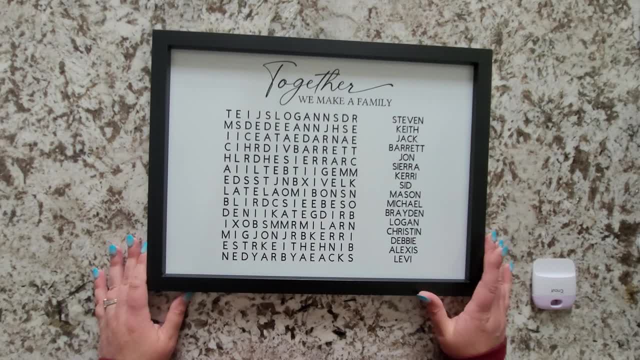 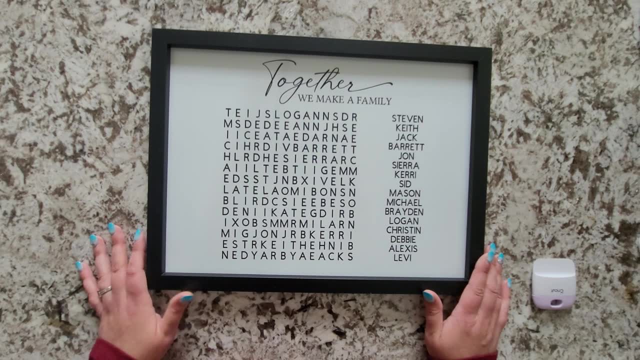 names over here and I forgot one of my mom's grandkids. There's a little girl named Bridget and I forgot to put her name on here, but there's a really easy way to fix it. So what I'm going to do is I'm just going to make another column right here and I'm going to write the word Bridget and 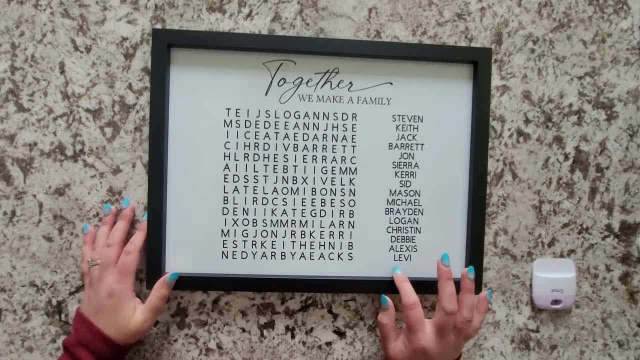 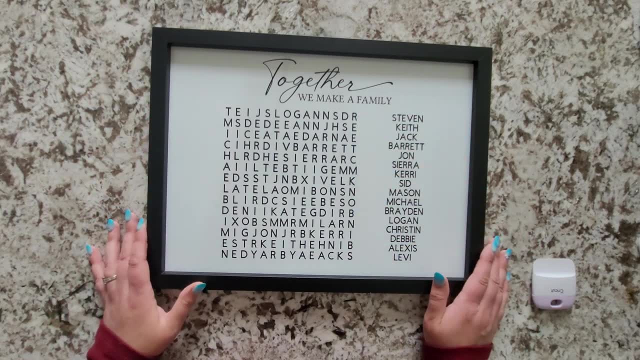 then I'm going to fill it in with some extra letters and then I can probably just squeeze her name down on the bottom. This is actually a really good idea to leave some space. So if you ever did want to add extra names, let's say you want to add some grandparents, aunts, uncles. 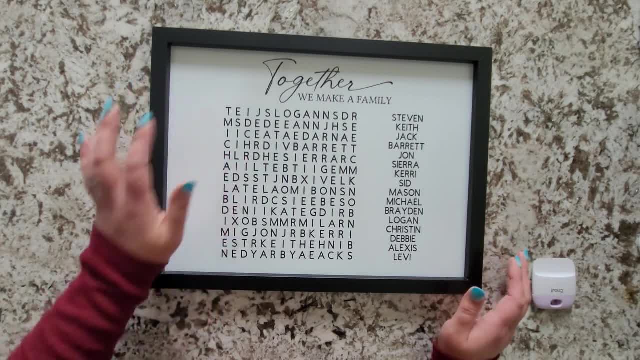 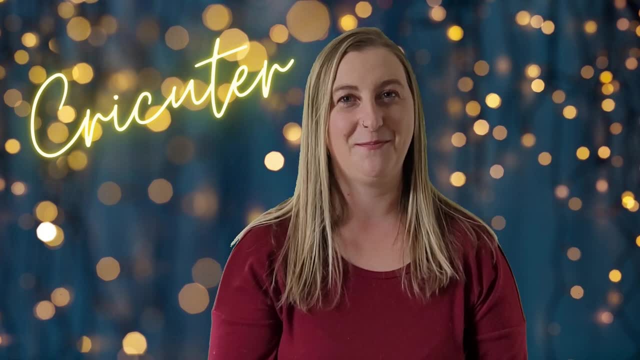 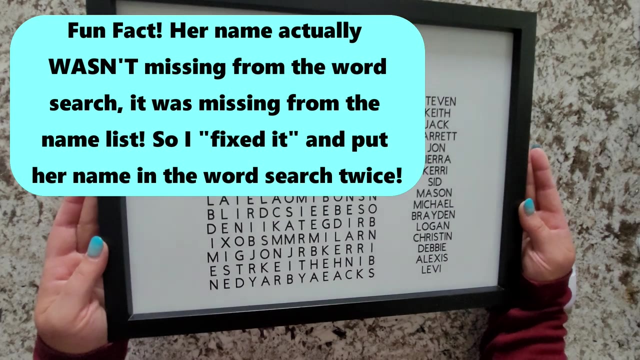 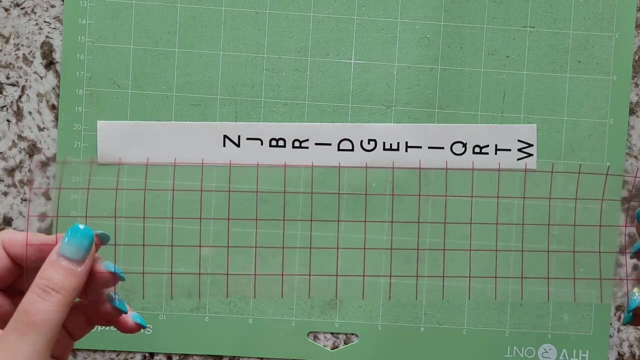 pets. there's a whole bunch of room on the side where you could do that. If you watch my Cricut channel, I mess up literally all the time, but I also show you how I mess up and I show you how I fix it, because almost every mistake that I make is fixable. Get yourself a thin piece of transfer.